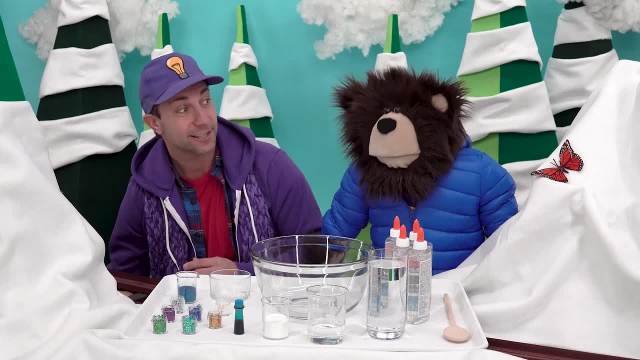 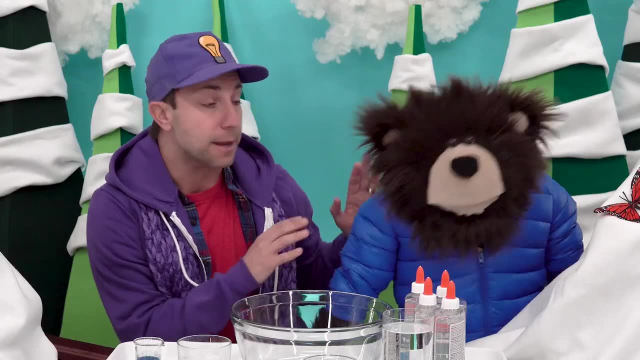 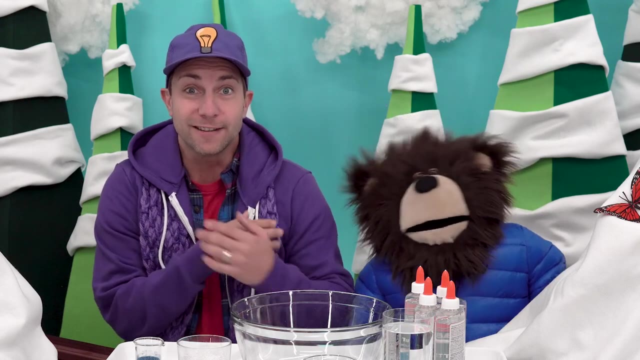 It's light blue, Mm-hm, Meta, look at all this snow. You have on a blue winter coat and I have on a purple sweatshirt and a purple scarf to stay nice and warm. Oh and look, Meta, We have a bunch of different. 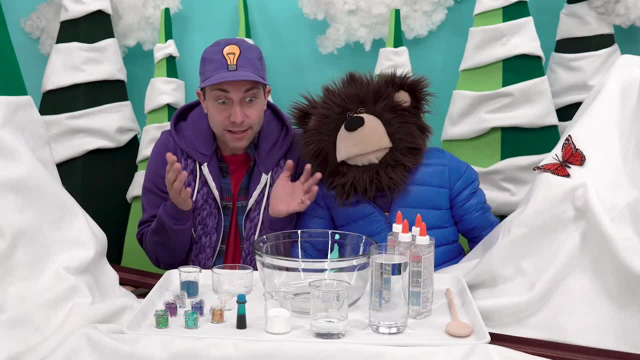 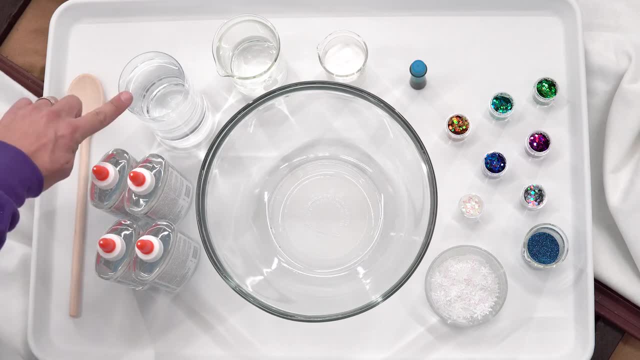 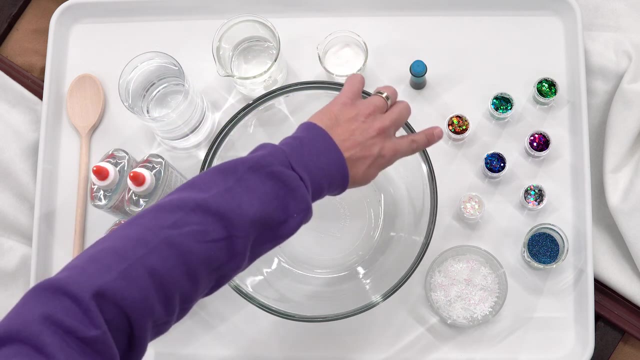 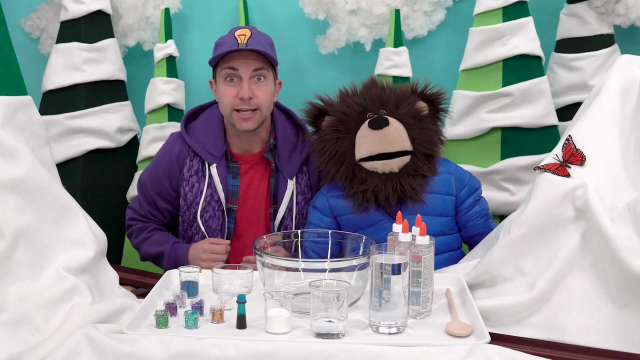 ingredients to do our winter slime science experiment. We have a wooden spoon, glue, water, contact solution, baking soda, blue food coloring, different kinds of glitter and confetti snowflakes. Are you ready to make some winter slime? Yes, 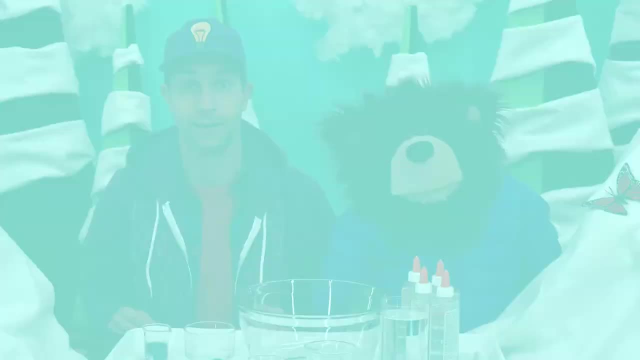 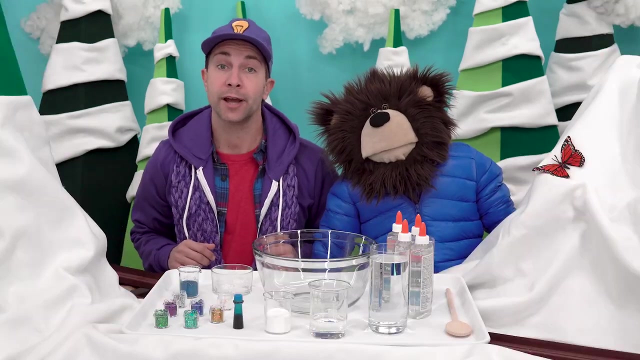 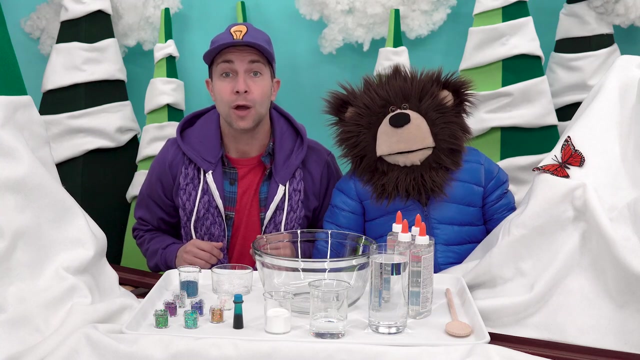 Okay, let's get started. So how do we make slime? Well, let me tell you, A chemical reaction occurs when you mix polyvinyl alcohol, which is found in our glue, with borate ion, which is made when you mix contact solution with baking. 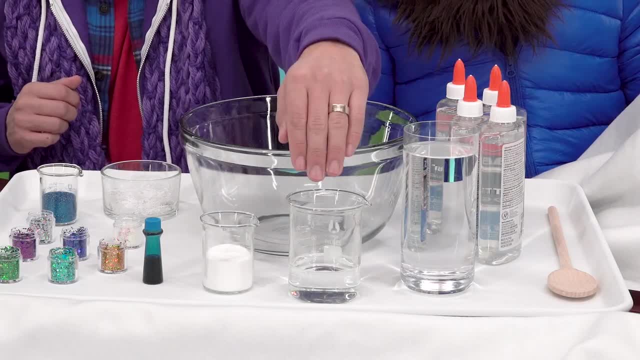 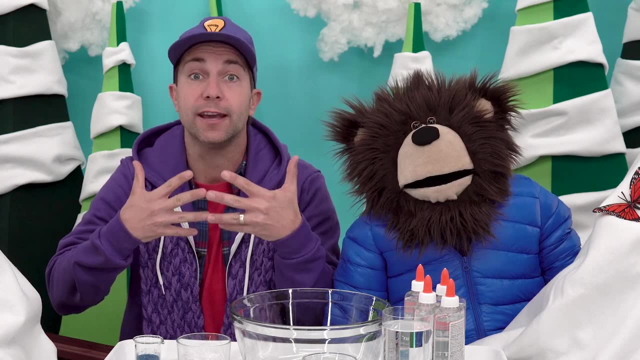 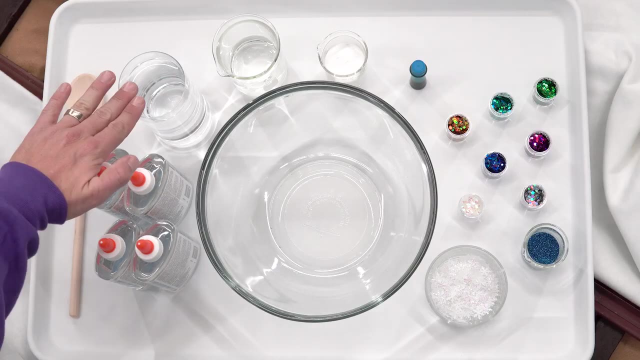 soda. When the glue, contact solution and baking soda are mixed, the molecules attract together or they combine, and the result is slime. Now, to avoid making really hard slime, we have to add water. Now, depending on how old you are, you may need a grown-up to help you mix everything. 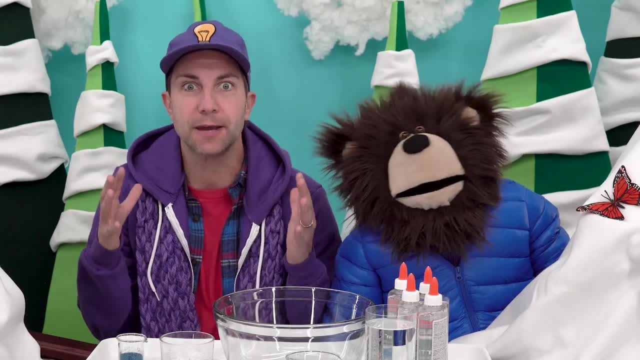 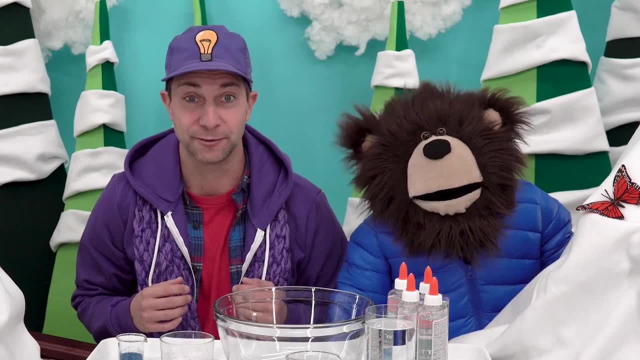 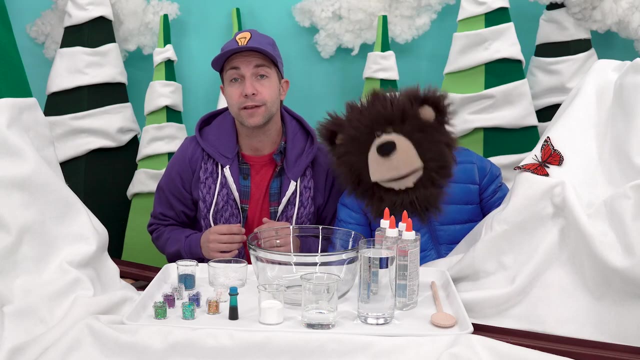 together, We are going to make a really big batch of slime today. so, grown-ups, if you are doing this at home, you may want to cut our measurements in half. In today's mix, we are going to use four large bottles of clear glue- approximately 36 ounces of glue. 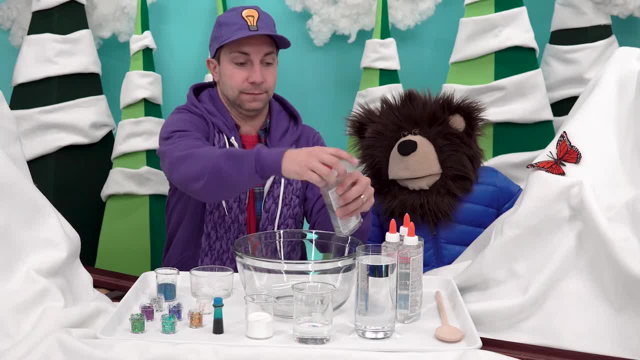 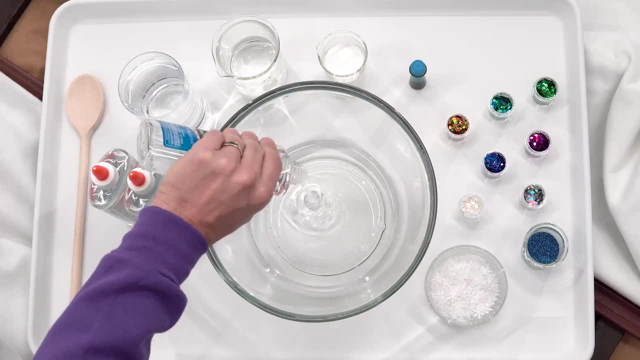 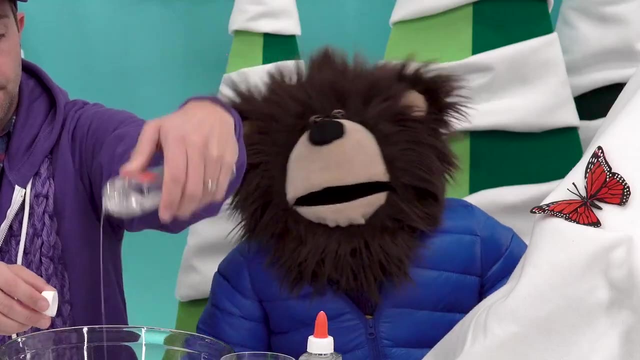 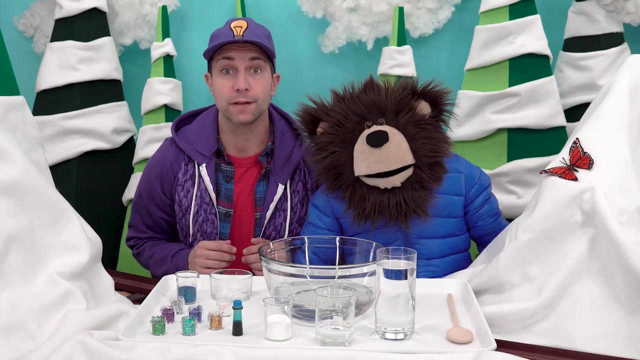 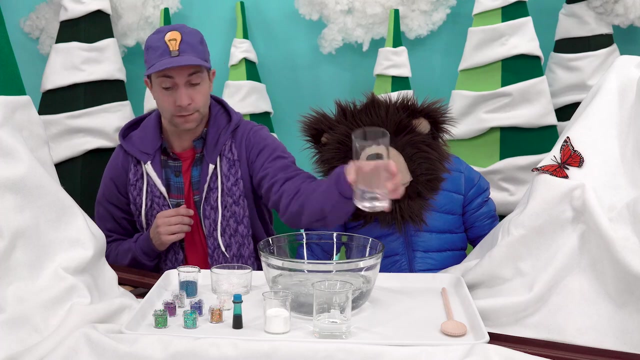 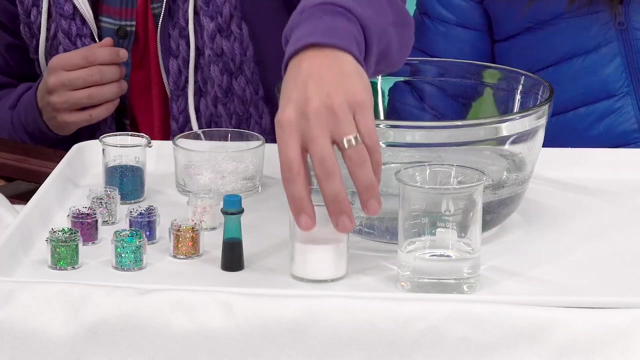 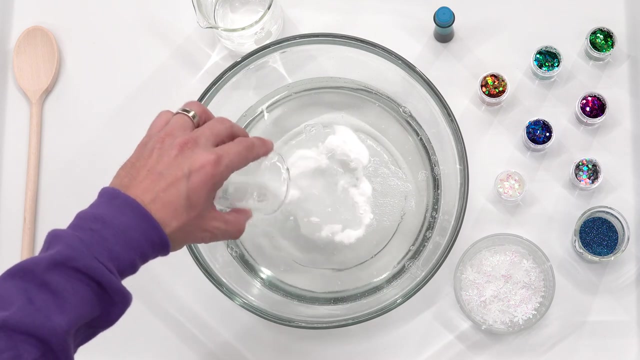 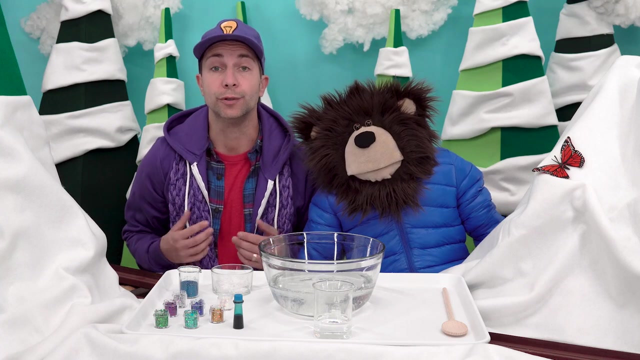 So let's do it. Next, we are going to add 16 ounces of water. Now we are going to add four tablespoons of baking soda. The next ingredient we are going to add is some blue food coloring- about four drops. 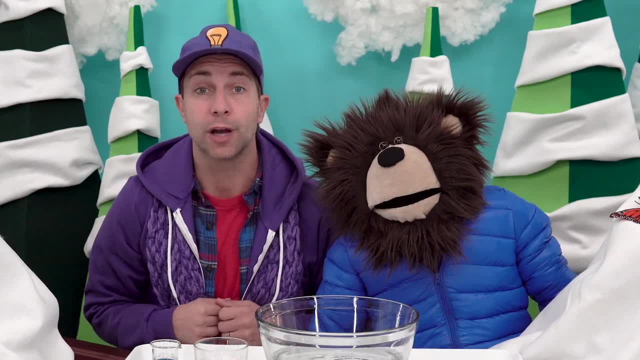 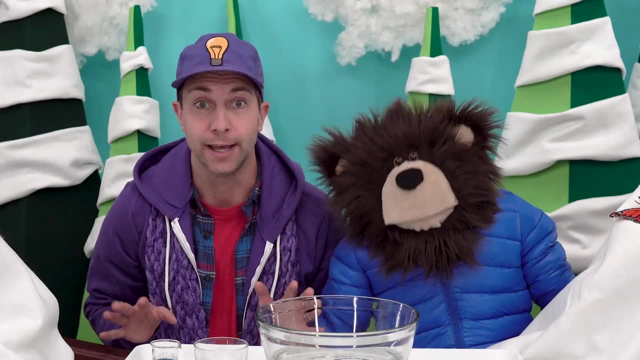 Now you can add whatever color of food coloring you want. I will just: deliciousl dieser. There is a really sweet glass bottle right there and we are going to put four tablespoons of the liquid soda in the glass. it could be green, red, yellow, whatever color you would like, because we are making winter slime. 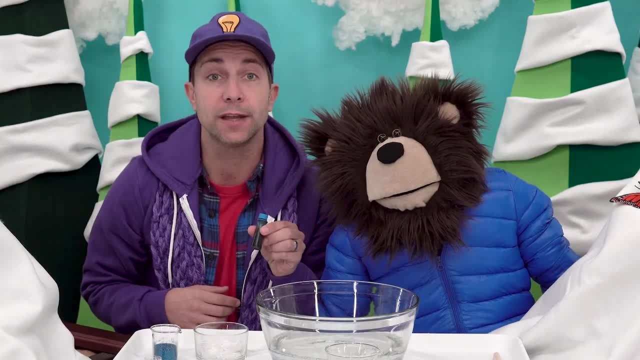 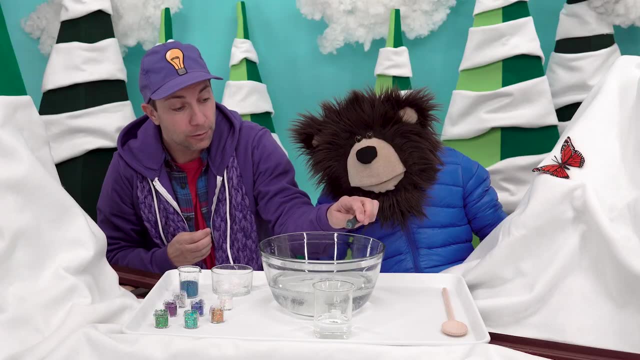 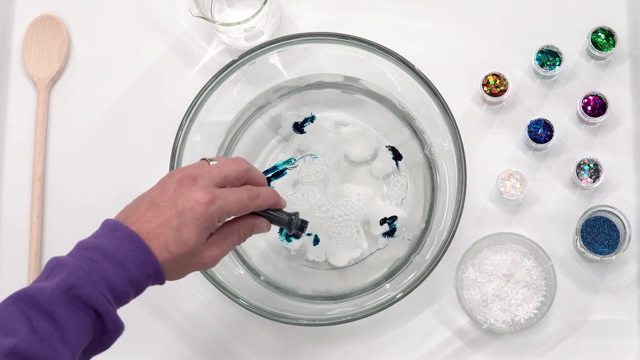 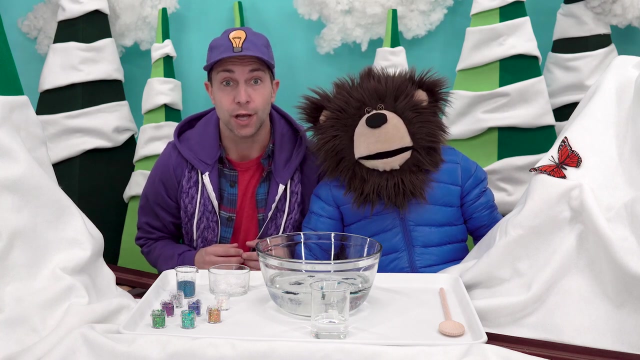 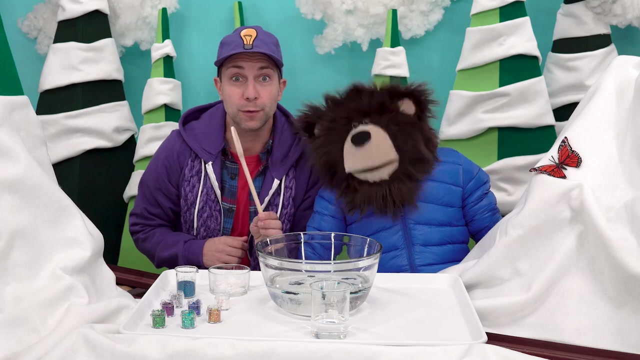 we're going to use the color blue to represent winter, ice and snow. all right, you ready meter before we add decorations and the contact solution. we are going to mix all of this together really well with a large wooden spoon. i'll say it again: it's really important that you 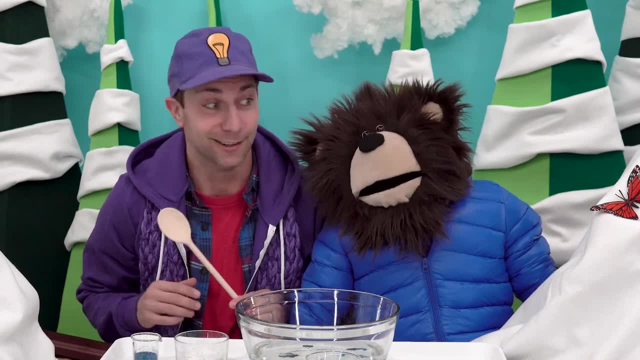 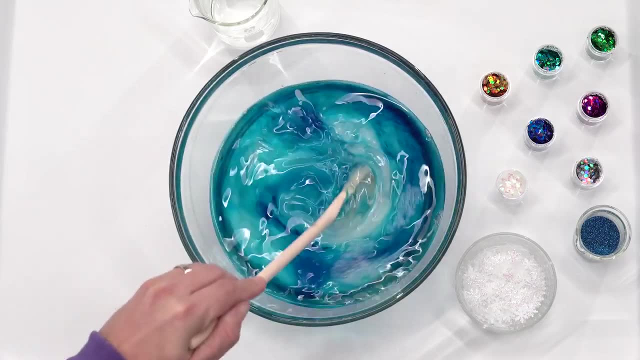 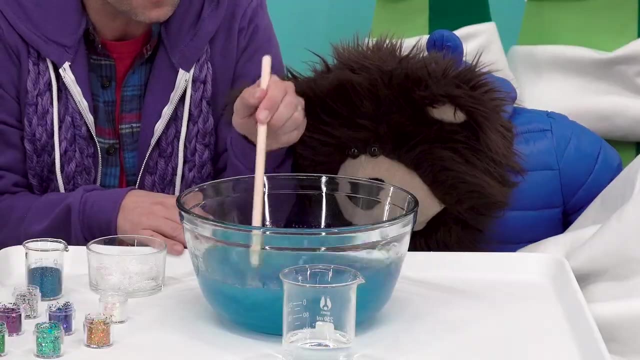 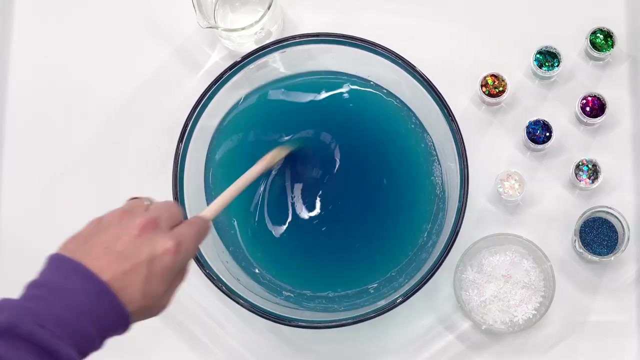 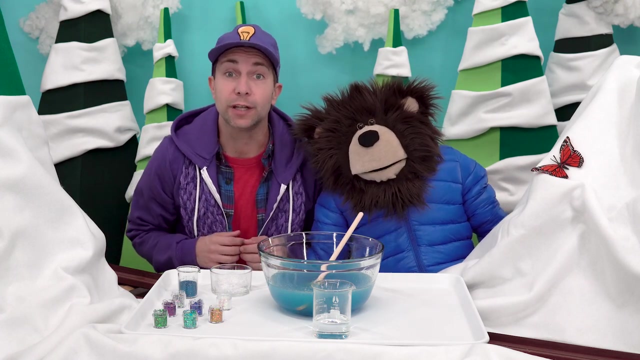 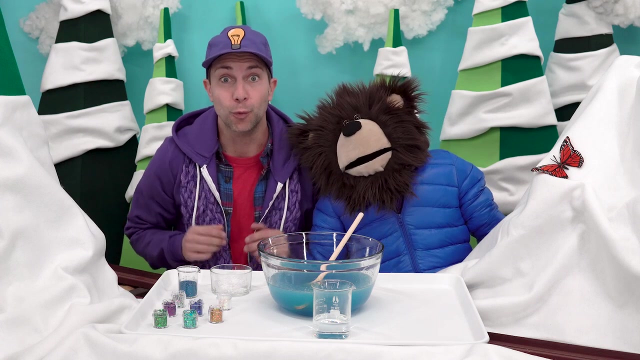 mix all of these ingredients really well. okay, all right, let's mix it together. look at that. okay, here is where the fun really starts to happen. we are going to add some blue glitter to our mixture and again, you can add any color of glitter that you want. all right, let's do it. 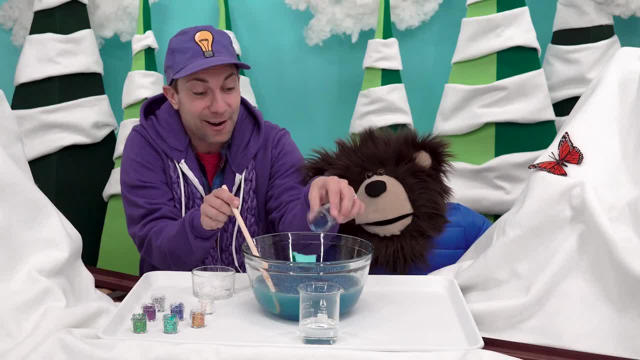 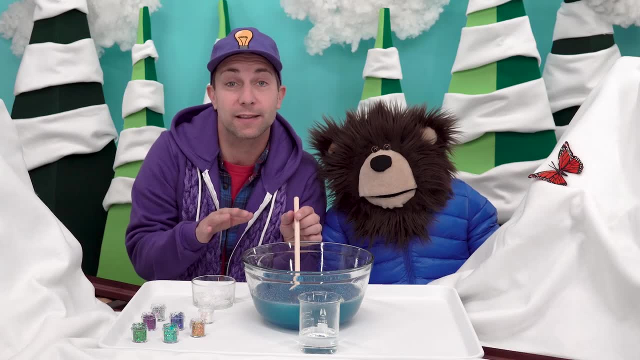 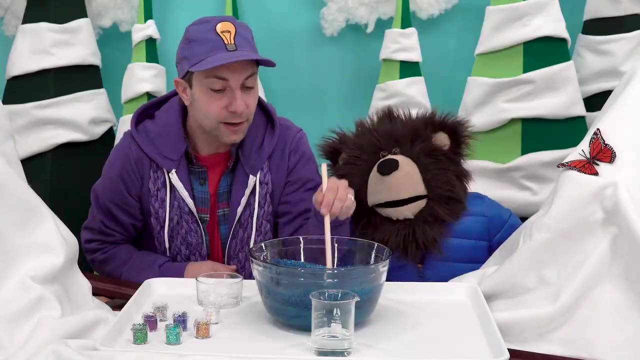 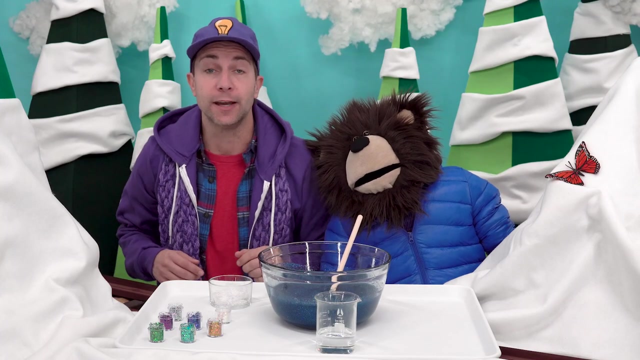 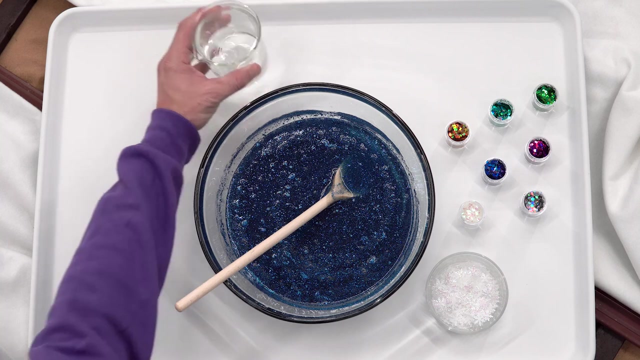 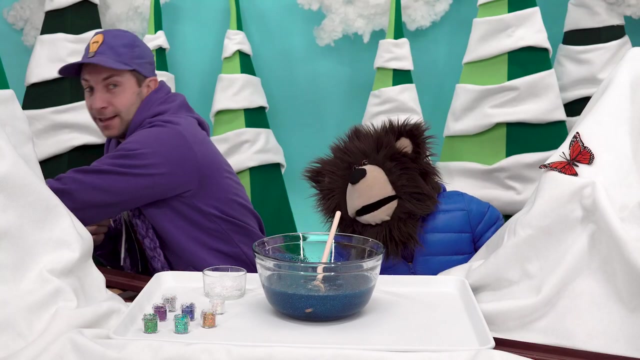 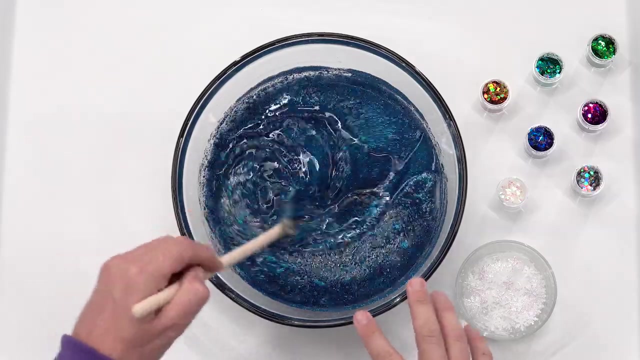 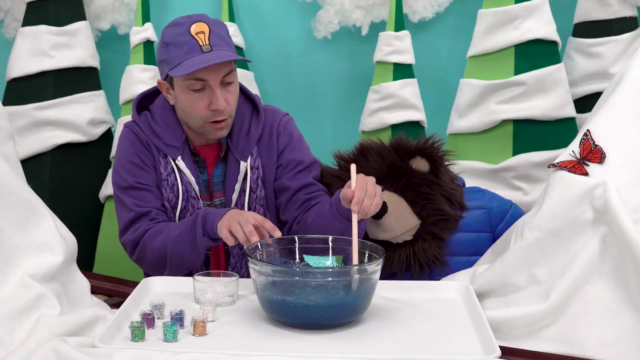 okay. so now we have to mix this really well again. okay, the last thing we are going to add is eight tablespoons of contact solution. are you ready? all right? okay, now we need to mix this together really really well. whoa, do you see that, mayta? oh, do you see what's happening? 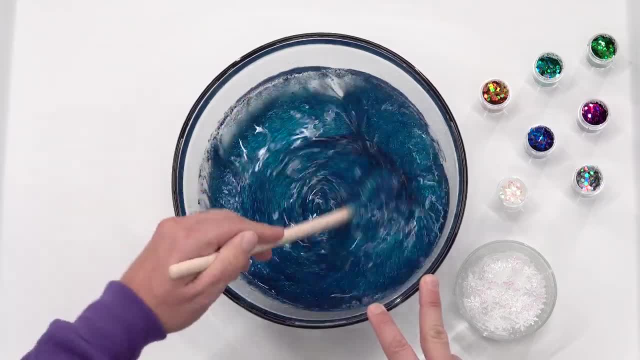 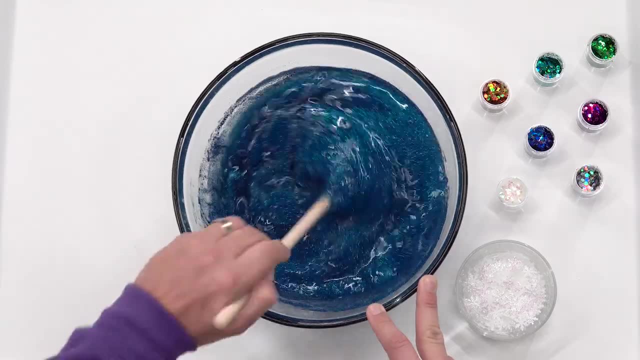 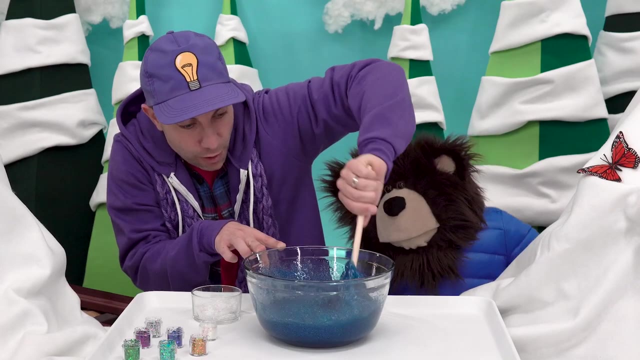 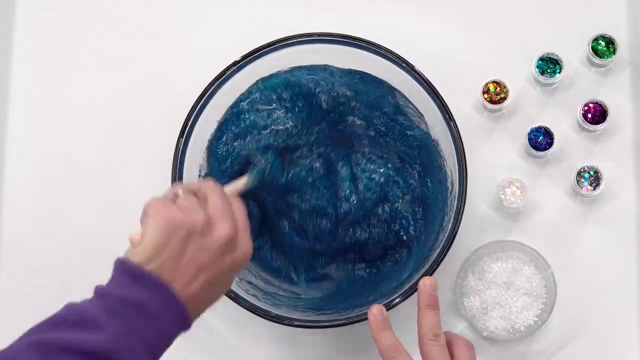 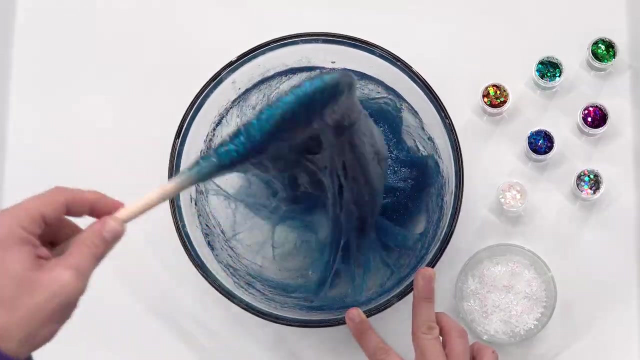 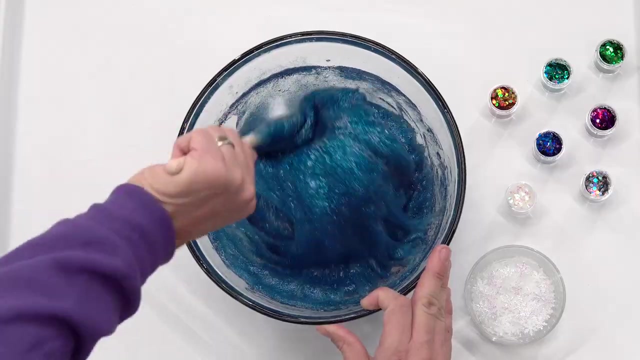 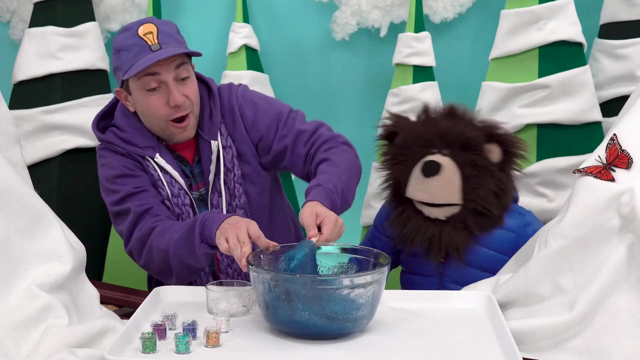 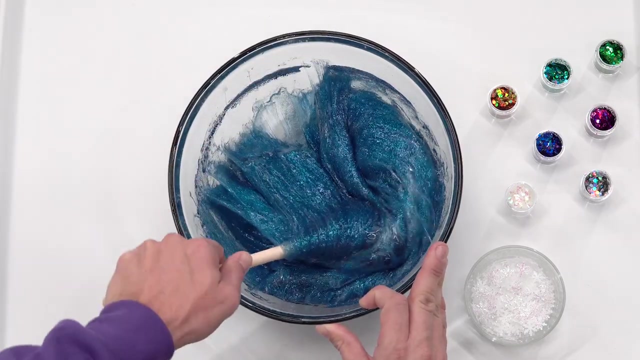 the glue, contact solution and bake in soda are starting to attract to each other and they are starting to form slime. whoa see that me? that's awesome. our slime is starting to really form. whoa okay, meita, i can do this me too. here we go. 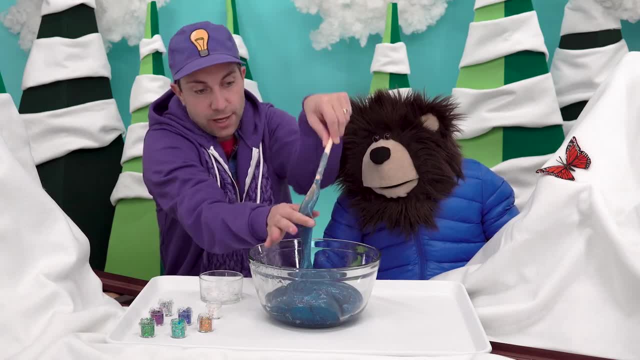 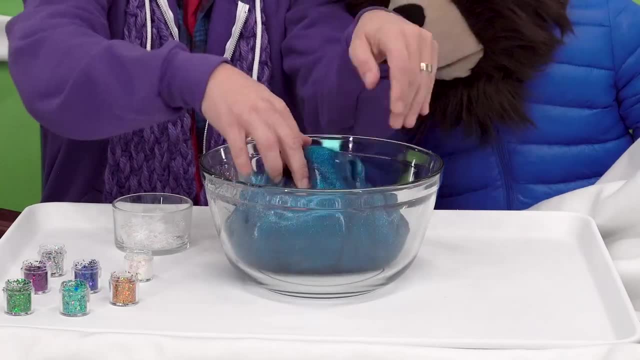 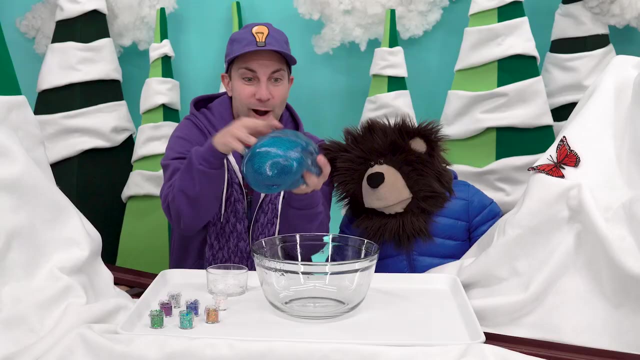 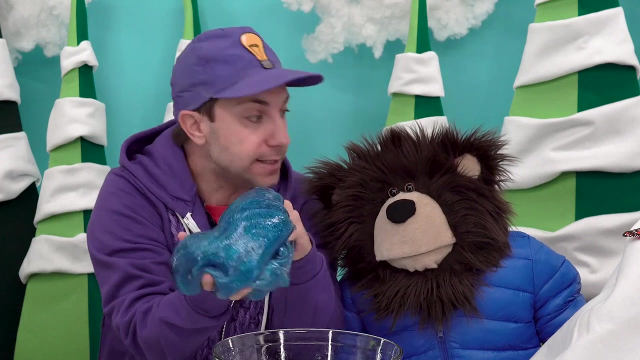 all right, meita, let's pull our spoon out of the slime and pick out our slime, the slime up, Whoa, You see this, Mayta, Look at that. Wow, Whoa. But wait, Mayta, We have to decorate our slime. 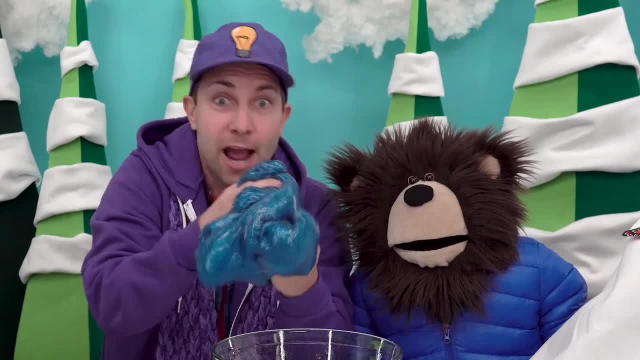 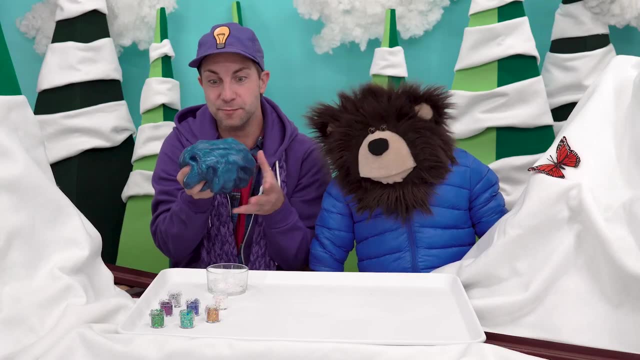 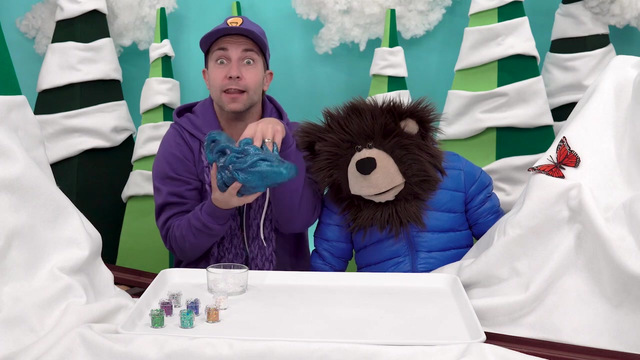 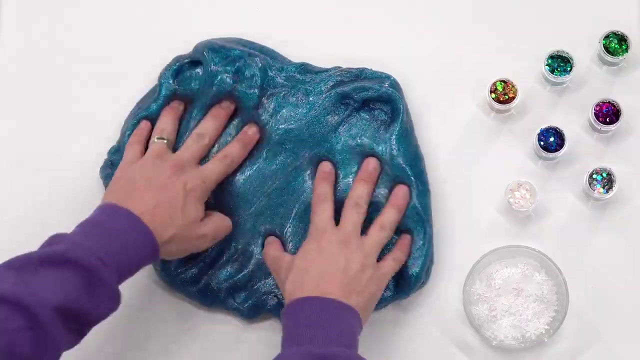 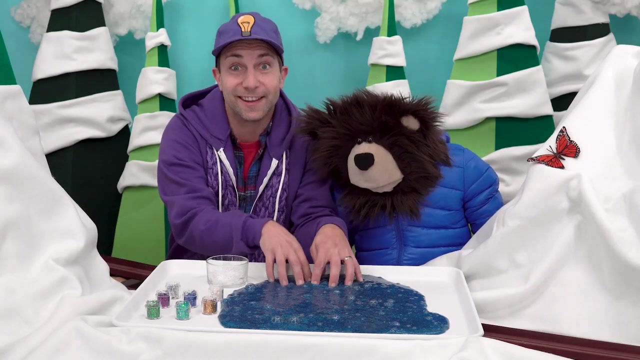 with chunky glitter and confetti snowflakes. Whoa, Okay, Before we decorate our slime, we have to spread it out on this white tray like this: Whoa, Look at that. Mayta, Okay, Mayta, This looks. 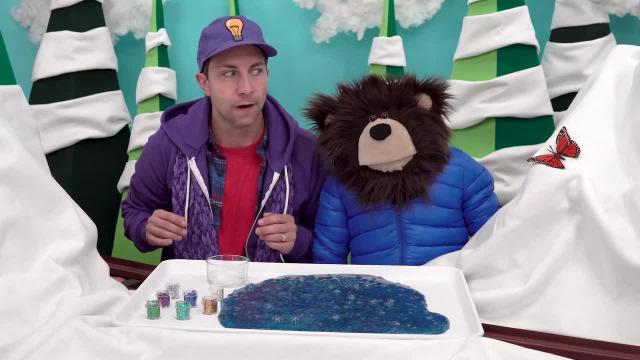 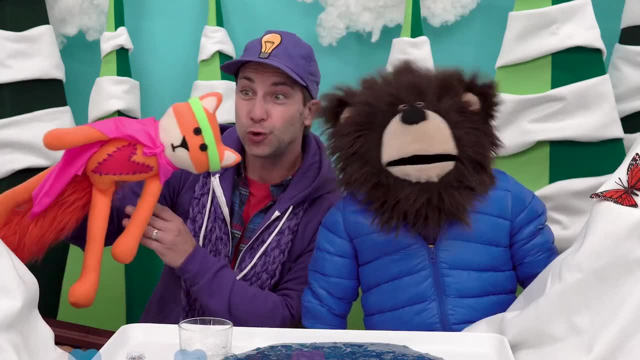 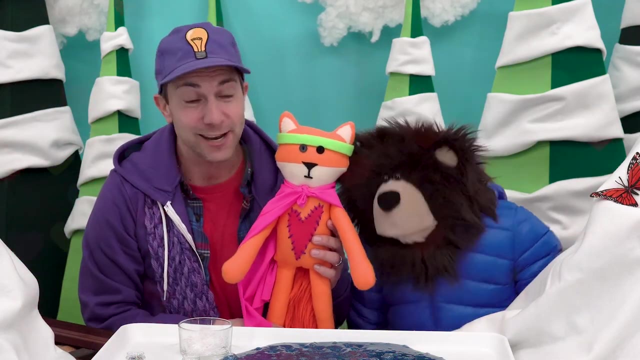 great. Wait, Do you hear that? It sounds like a superhero is flying. It's flying through the air. Oh look, It's Mayta's favorite stuffy, Mimi, the Orange Fox. What, Mimi? I bet you are here to help us add. 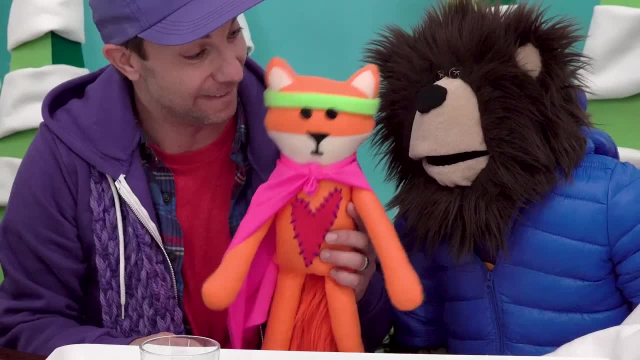 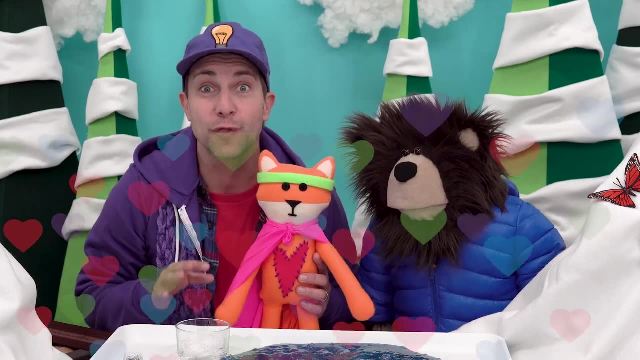 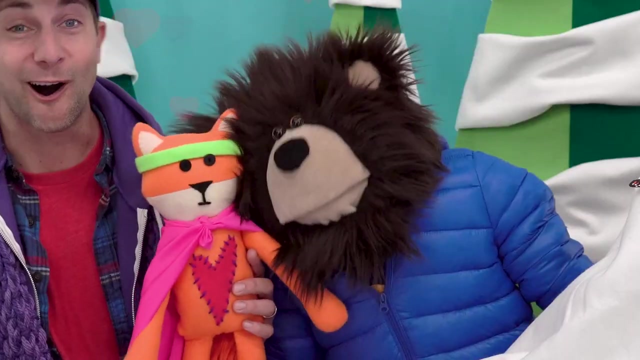 chunky glitter to our winter slime. I knew it. Mimi's superpower is spreading kindness all over the world. Mimi, that is very kind of you to help us. Aww, Okay, So Mimi is going to add light, blue, chunky glitter. 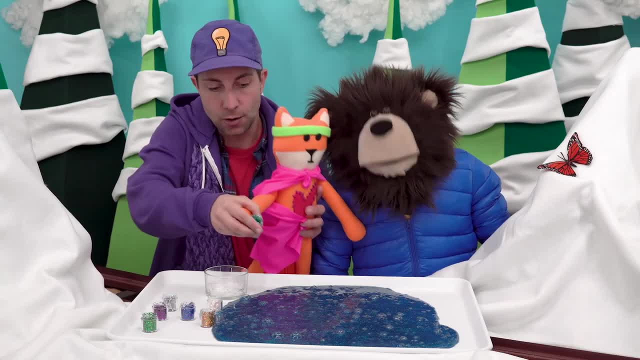 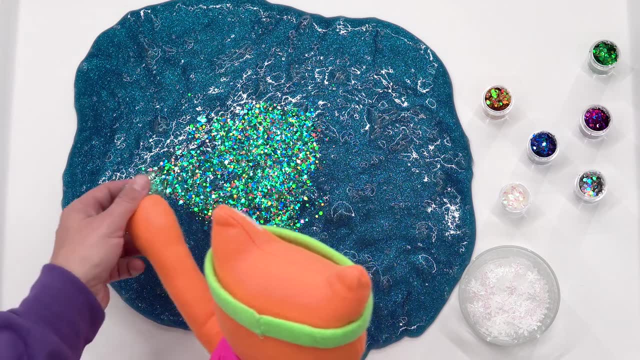 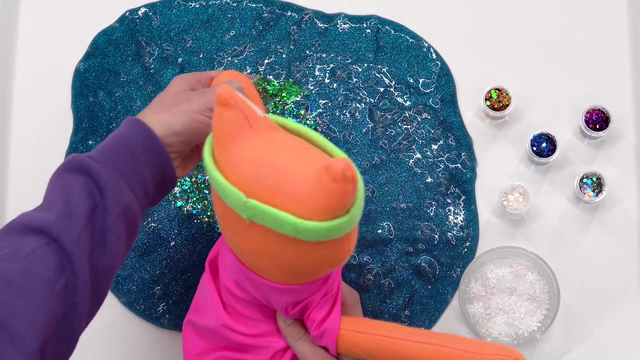 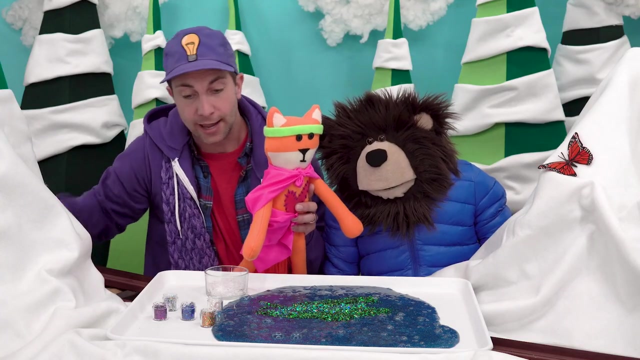 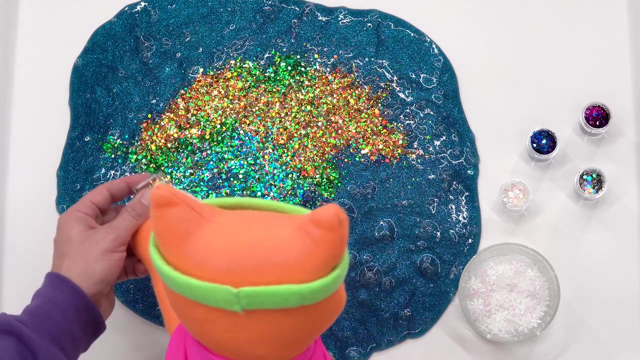 Get that for you, Mimi And Whoa. And some green chunky glitter- Whoa. Ooh, There you go. Okay, There you go. and some gold chunky glitter- whoa. That looks really cool, Mayta. 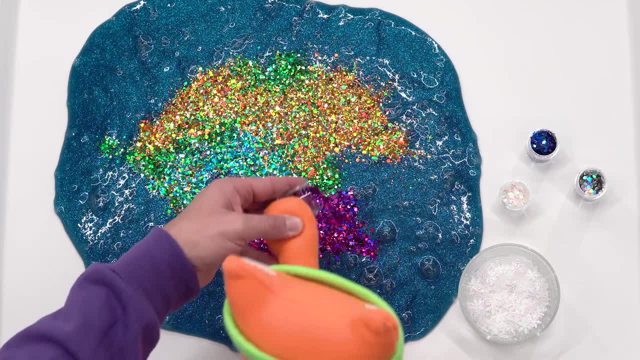 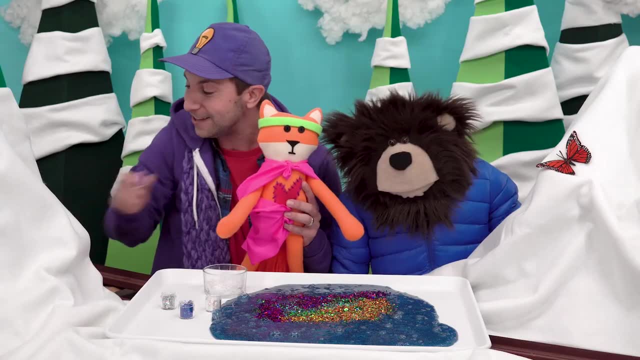 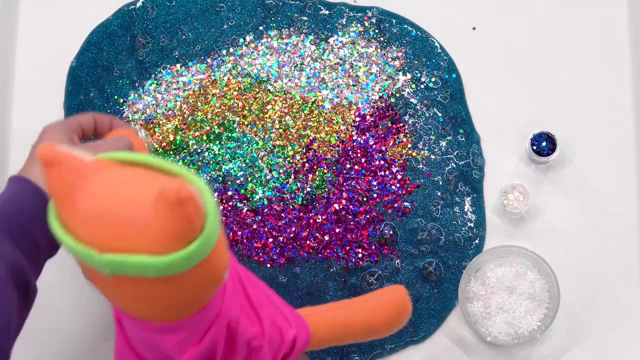 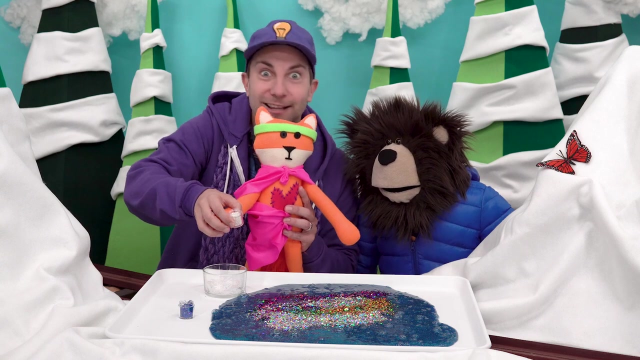 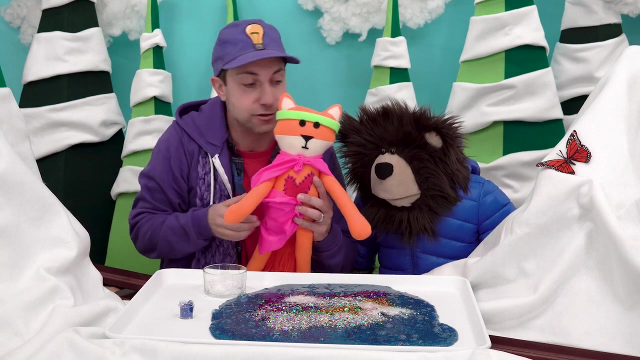 And some purple chunky glitter- whoa- See that, Mayta, Mm-hmm. And some silver chunky glitter- whoa. And some white and pink chunky glitter- ooh, Oh, and the last chunky glitter Mimi is going to add. 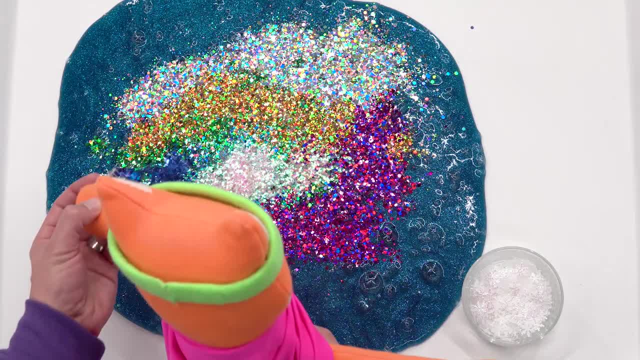 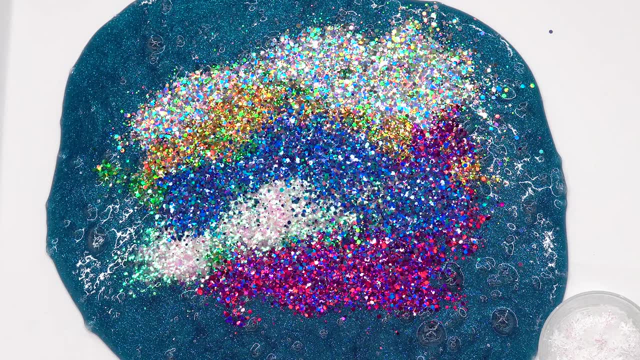 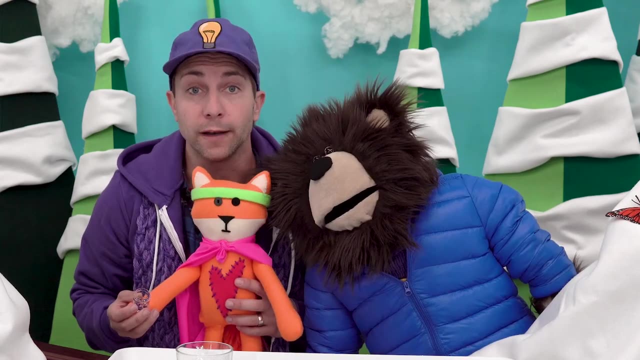 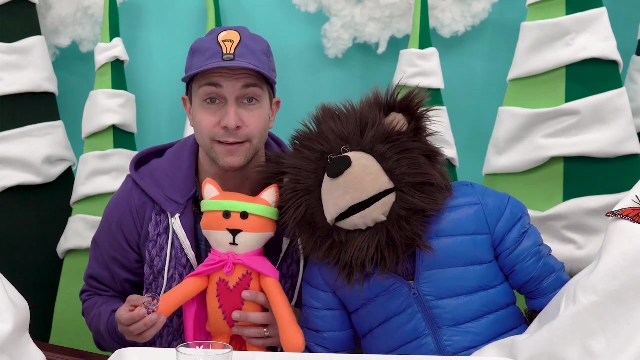 is some blue right on the top. whoa, Wow, that looks really neat and very cool, Colorful. I'll say it again: You can add whatever decorations you want: Sequins, puff balls, whatever you want. It does not need to be the same as mine. 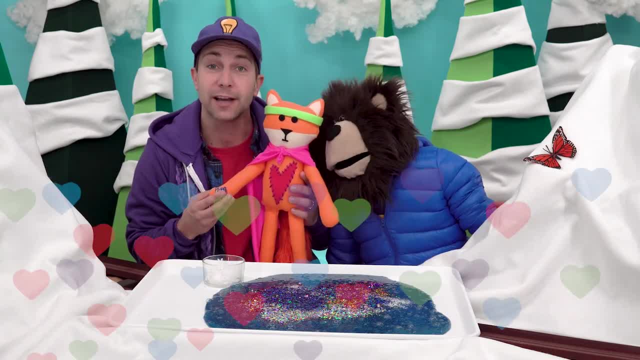 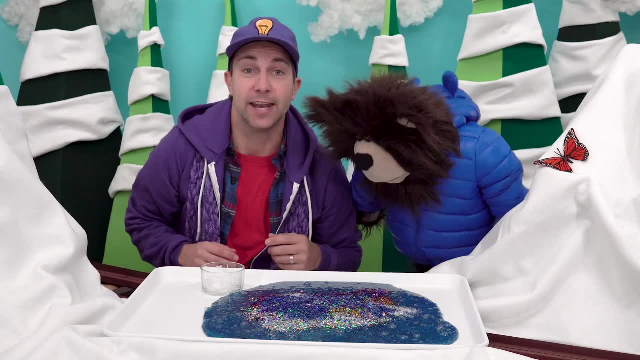 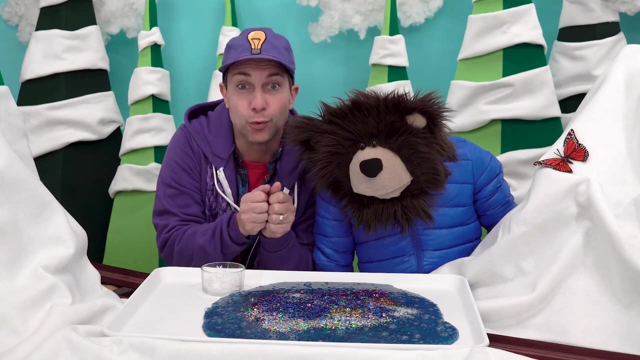 Thank you again, Mimi, for your help. That was very kind of you. Bye, Mimi. All right, the next step we are going to do is fold our slime over our glitter and mash it up really well so that we mix the glitter into the slime. 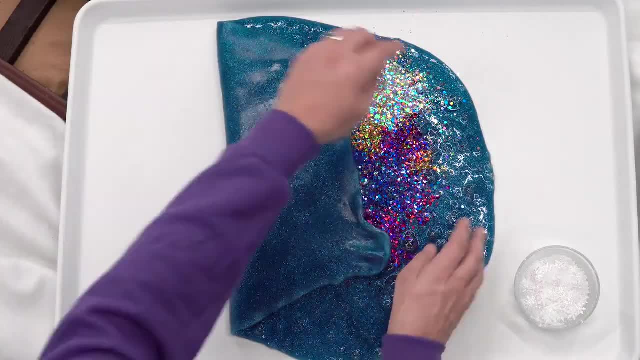 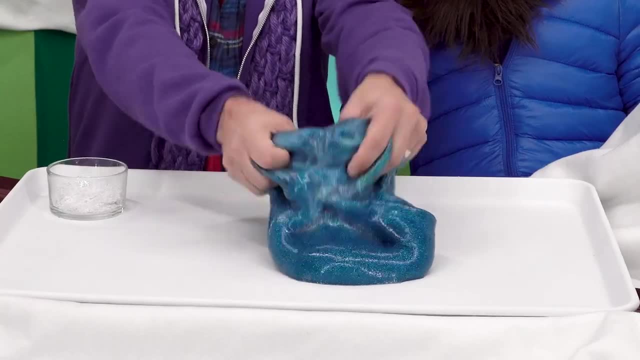 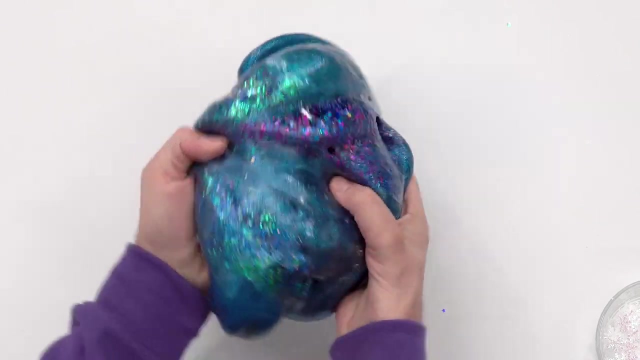 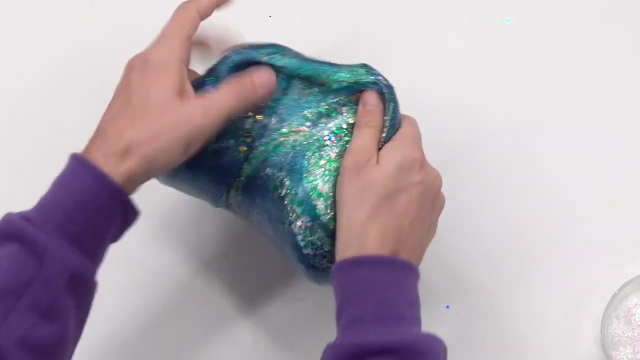 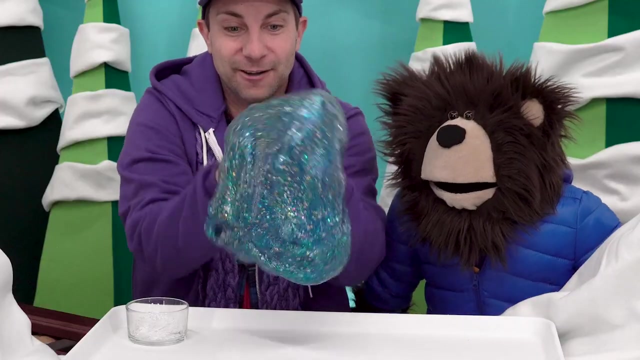 Are you ready? Mm-hmm. Okay, We folded the slime, Now let's mash, Whoa, Mash and mash. See that, Mayta, The glitter is starting to really mix, And now we're going to add the slime into the slime. 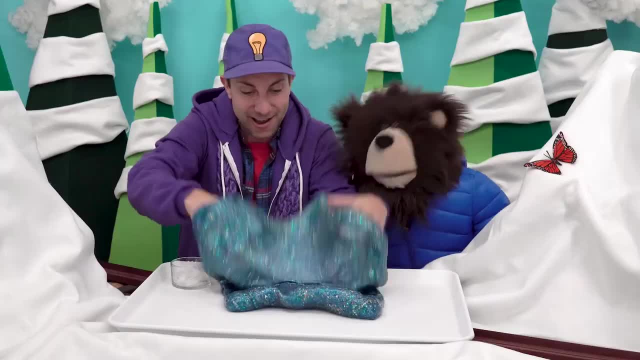 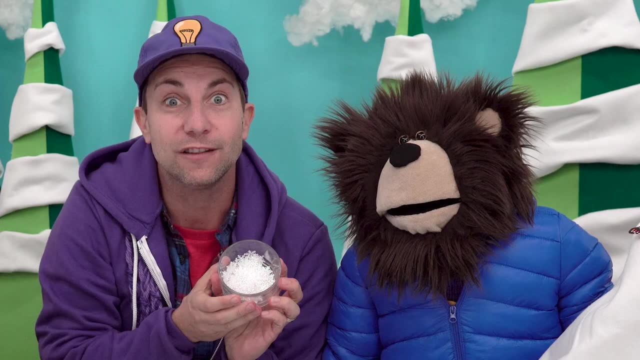 Whoa Mm-hmm. Wow, look at that. Whoa Mm-hmm. Okay, now the last decoration we are going to do is add some confetti snowflakes. Mm-hmm. Are you ready? 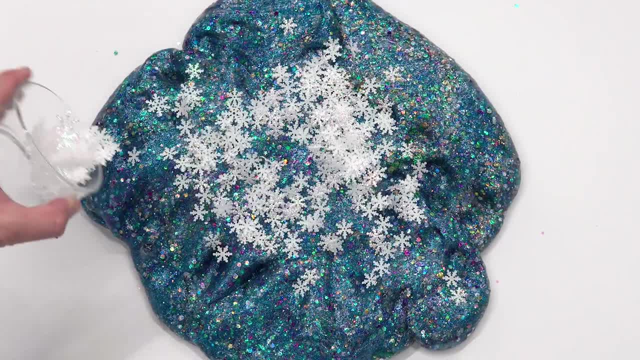 Mm-hmm. All right, here we go. Whoa, look at that, Mayta, It's snowing, Mm-hmm, Mm-hmm, Mm-hmm, Mm-hmm, Mm-hmm. 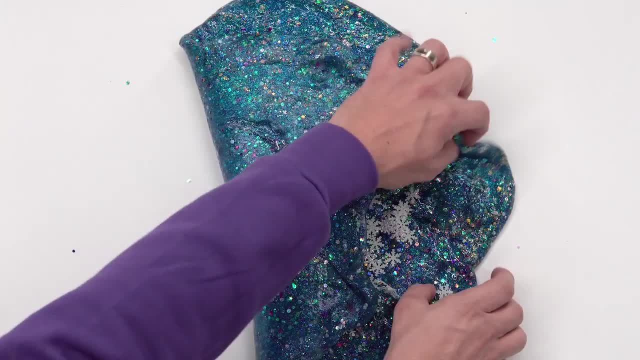 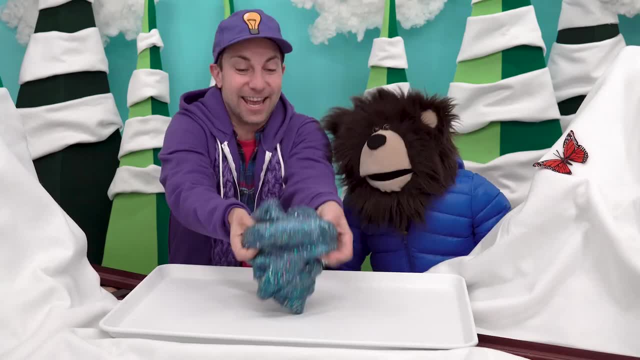 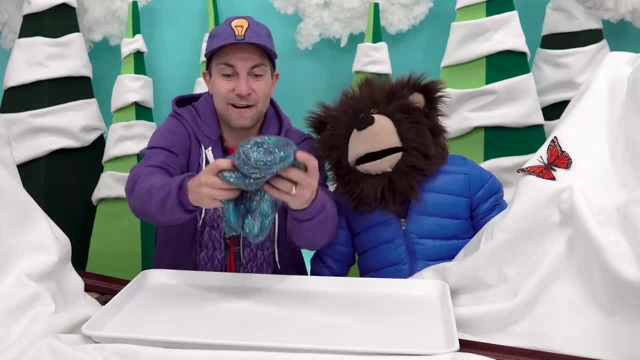 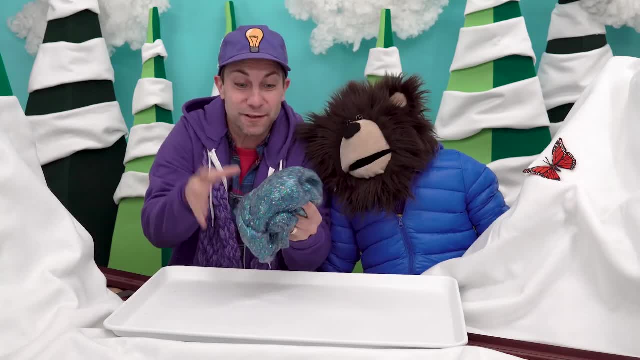 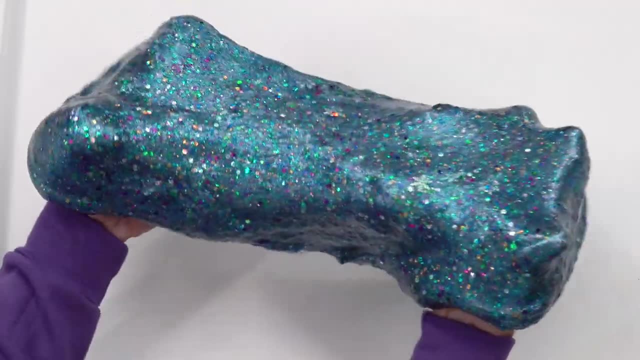 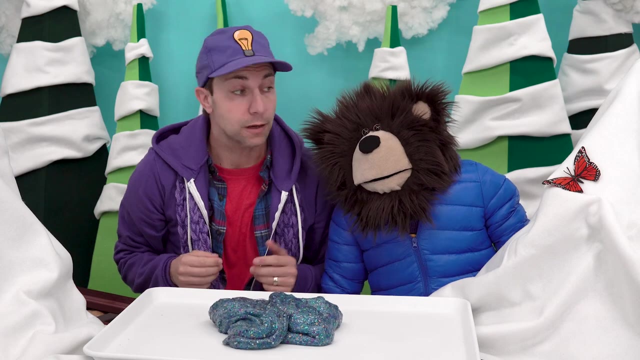 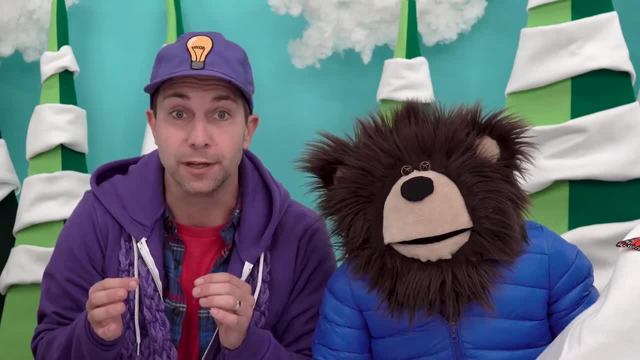 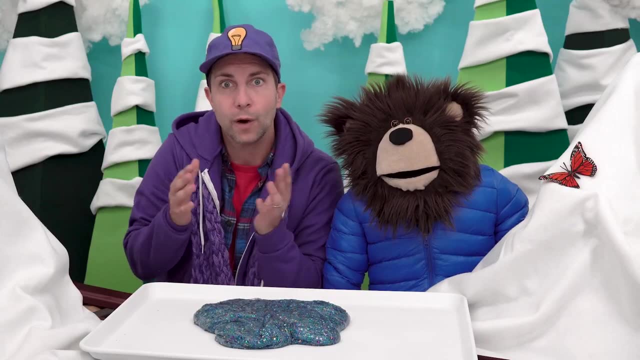 I'll tell you, Slime is a very special kind of liquid called non-Newtonian fluid, Mm-hmm. That means it's neither a solid or a liquid. In a way, Mayta, it's kind of both Mm-hmm. 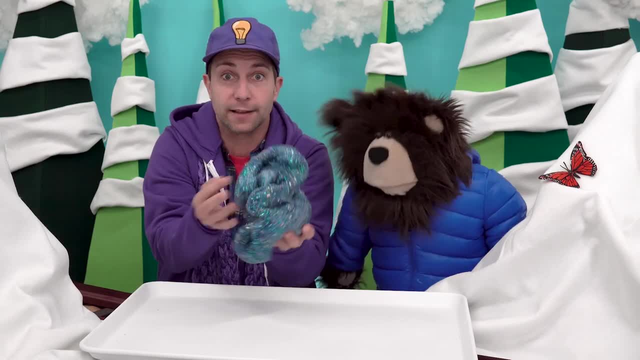 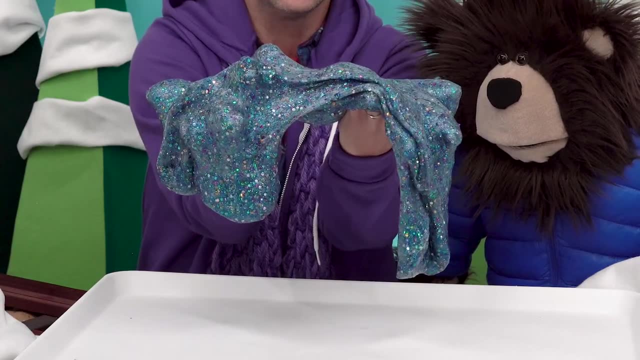 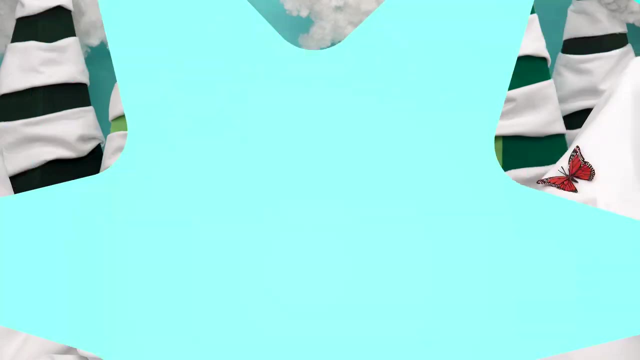 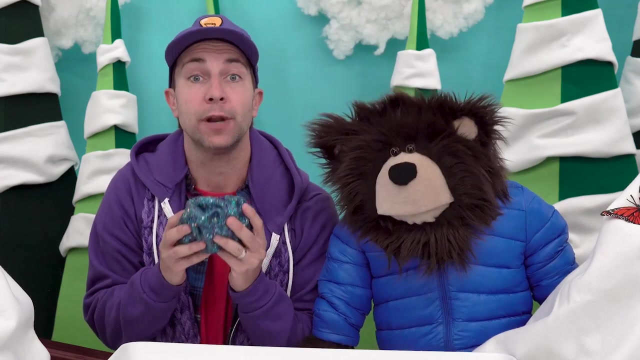 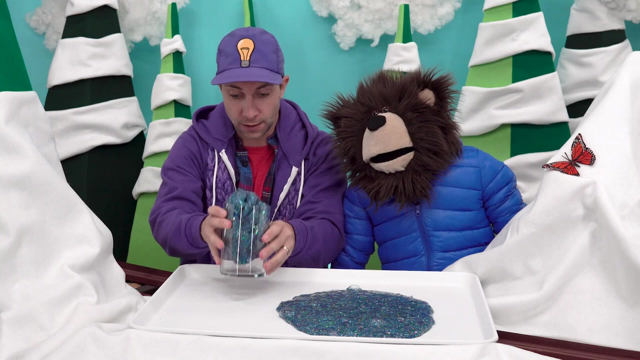 See, You can pick up slime like a solid, but the slime can also slide through your fingers like a liquid. another really cool thing about slime is that it does not have its own shape. see, when i put the slime in this glass jar, it takes the shape of the jar. 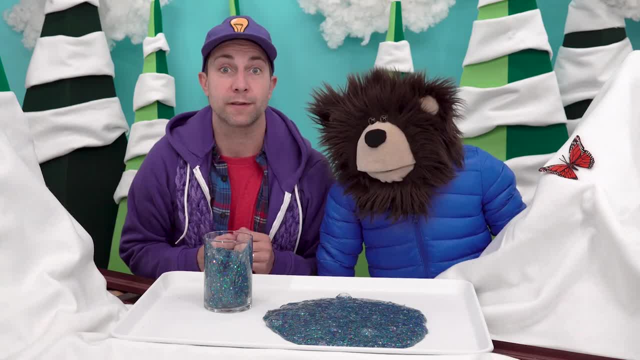 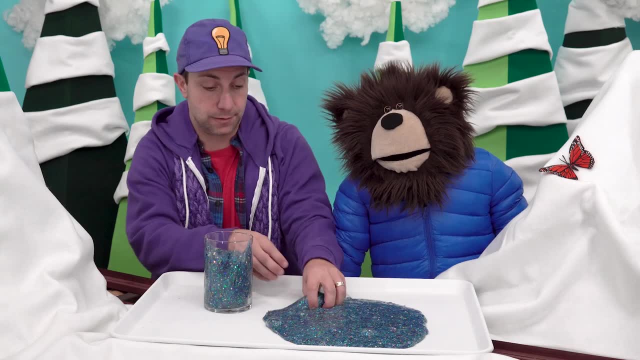 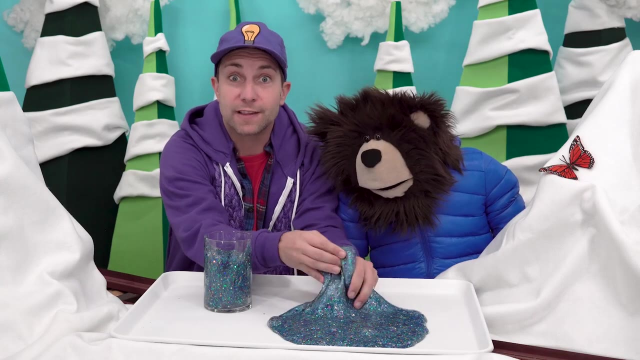 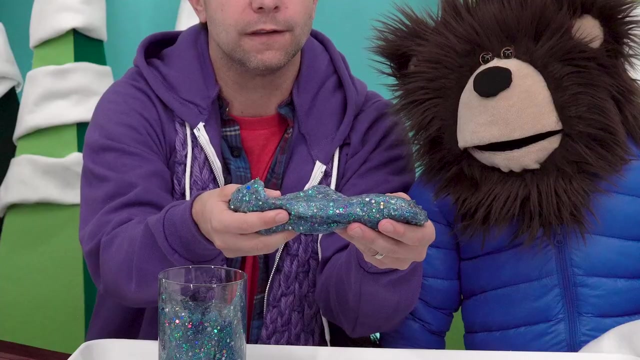 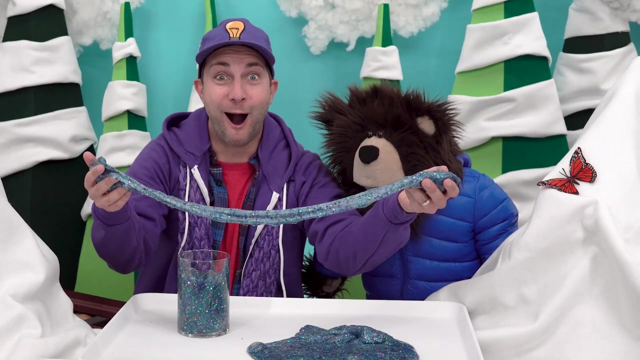 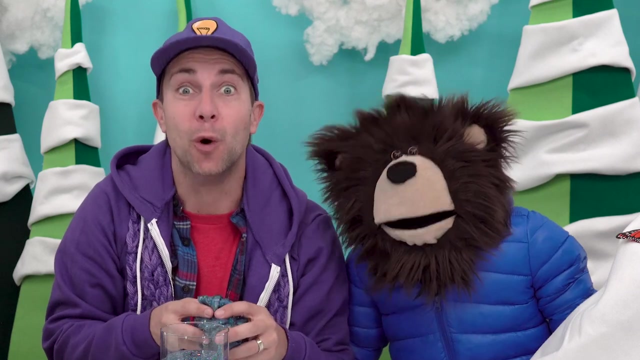 oh, now here's something really cool about slime. if i apply pressure or force to the slime and pull it fast, it will snap like this. but if i am gentle with the slime and pull very slowly, it will stretch like this. see that? whoa, that is really neat. there are so many fun things you can do with slime. 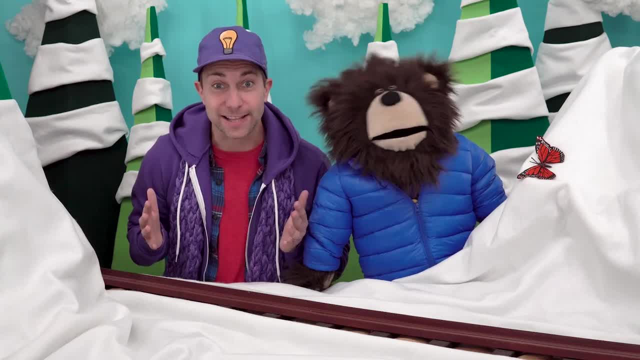 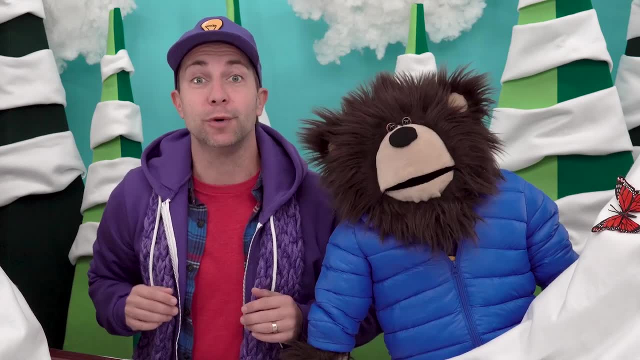 do you know what time it is? it's time to dance. this is where we stop what we are doing. stand up and dance. you can do whatever dance move you feel like doing. oh, do you hear that? it's the end of the video. thank you so much for watching and i'll see you in the next video. bye, bye. 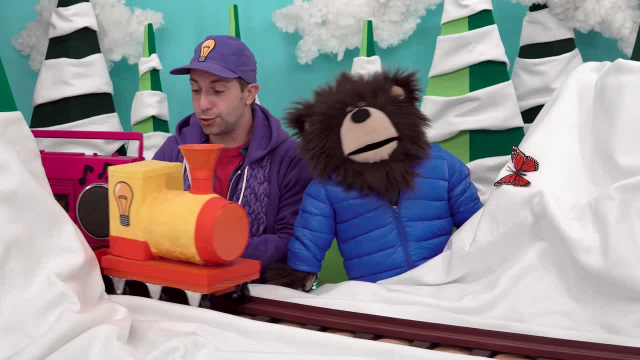 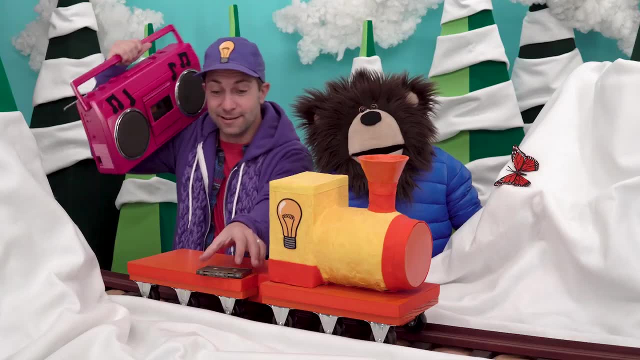 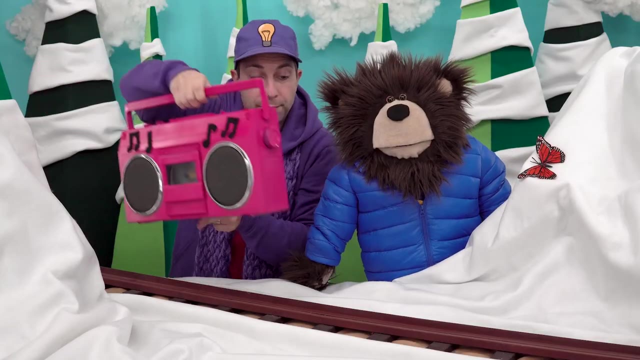 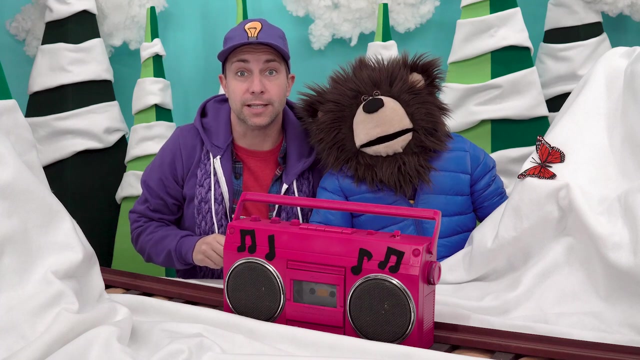 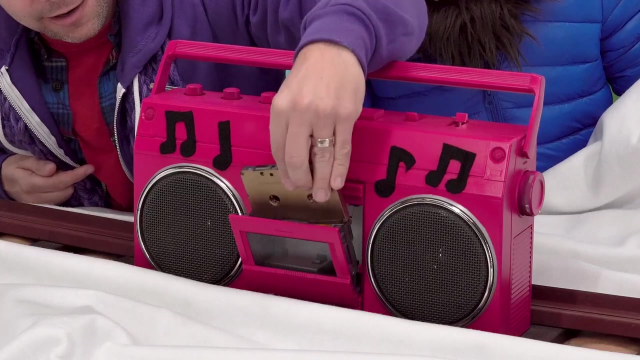 train and look, it's pinkie the boom box. hi, pinkie the boom box. all right, thank you, idea trading. okay, we will put pinky right here. pinky plays our music. i'm going to take this gold cassette tape and put it in here, then I will close it up and then I'm going to push the button with the. 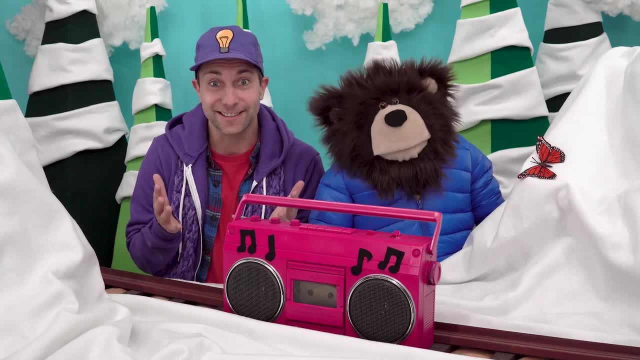 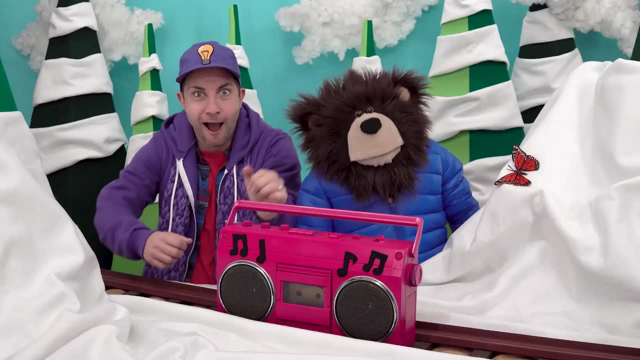 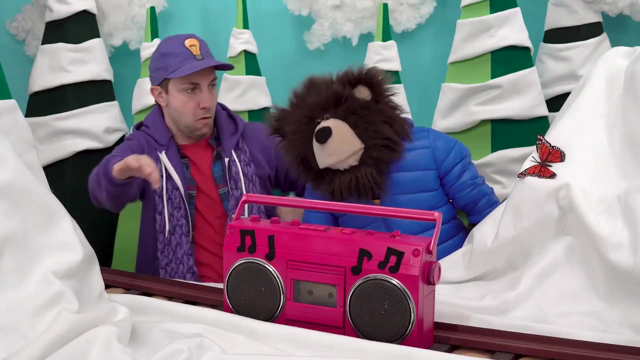 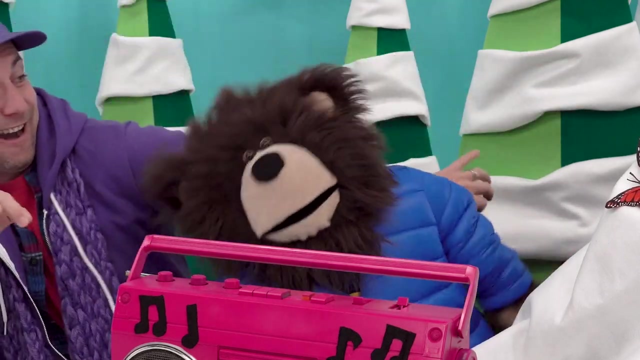 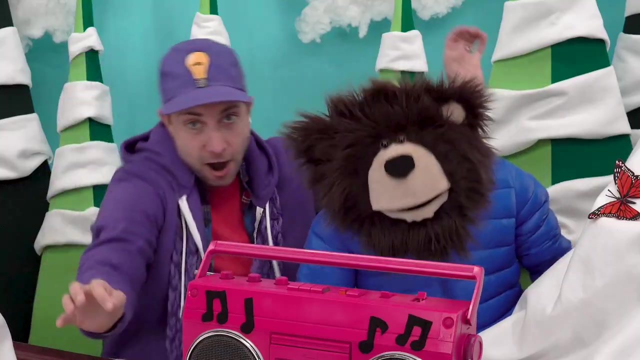 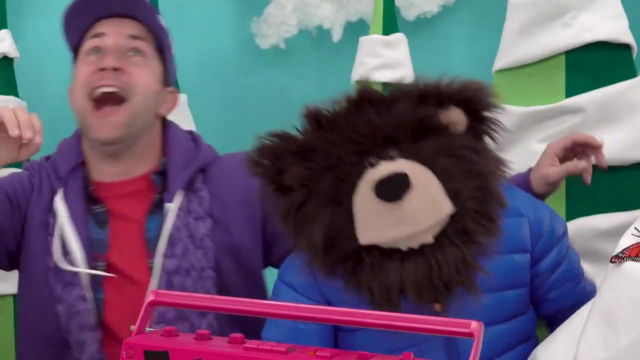 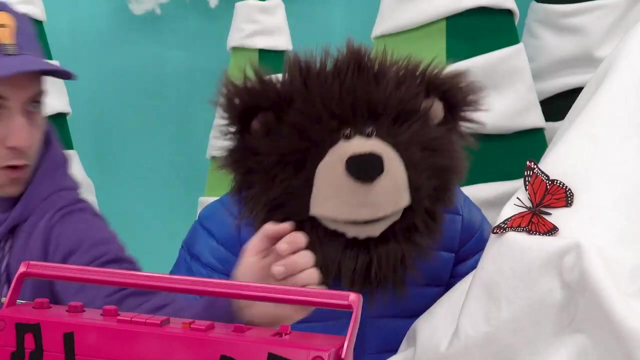 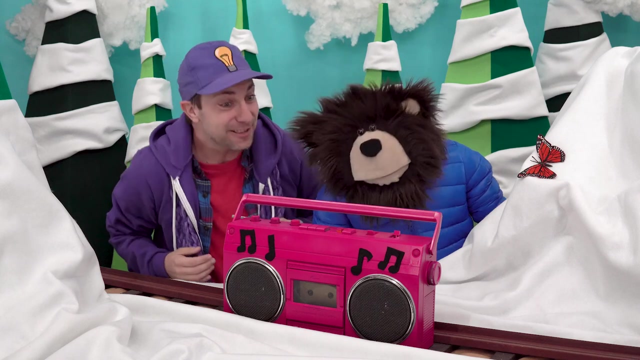 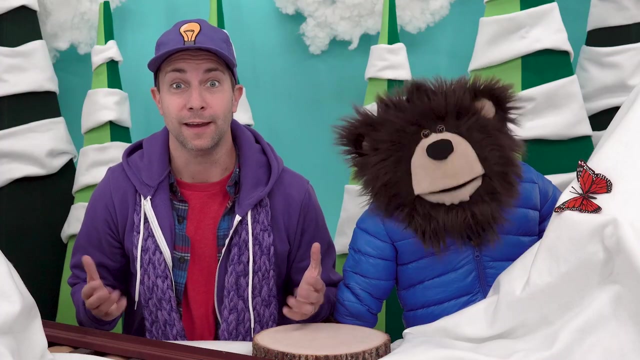 triangle on it, the play button. oh, are you ready to dance? yes, okay, I'm going to push the play button now. whoa, that was a sterisk dance, lot of fun. okay, let's get back to what we were doing. guess what? it's time to share some mate art. 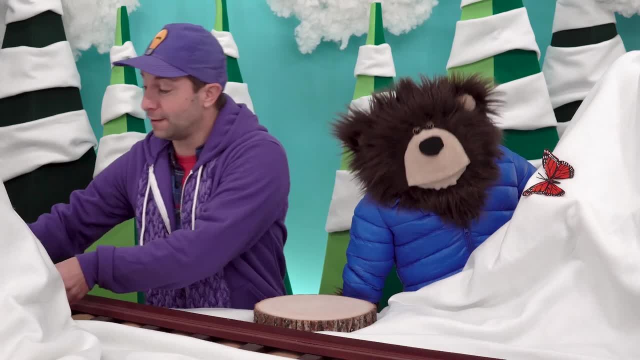 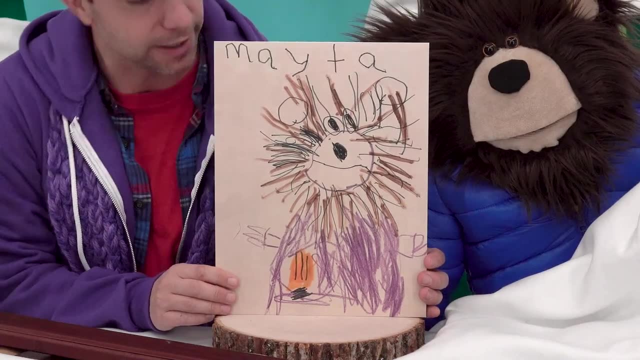 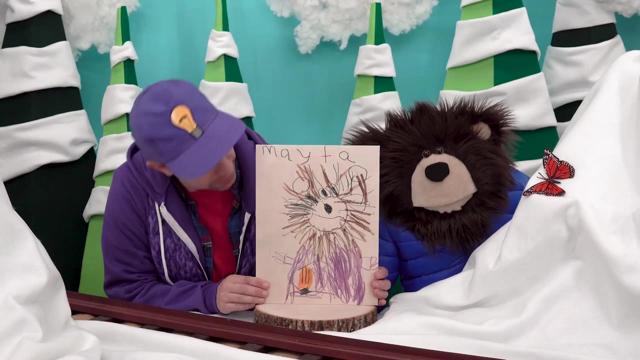 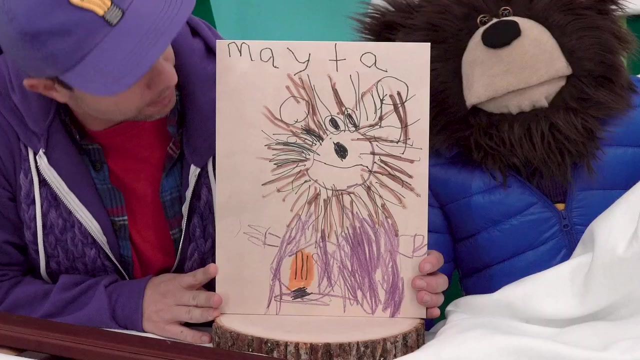 are you ready for our first piece of art? this artwork was sent to us by a family who lives in the united kingdom. an awesome kid named atreyu made this art mate. there you are right in the center of this. atreyu did an excellent job at coloring made to brown and coloring his sweater purple, and i really 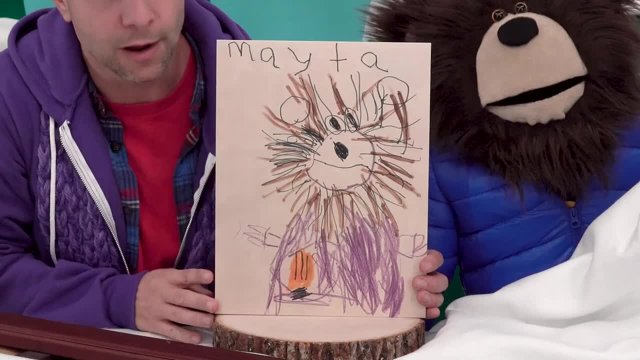 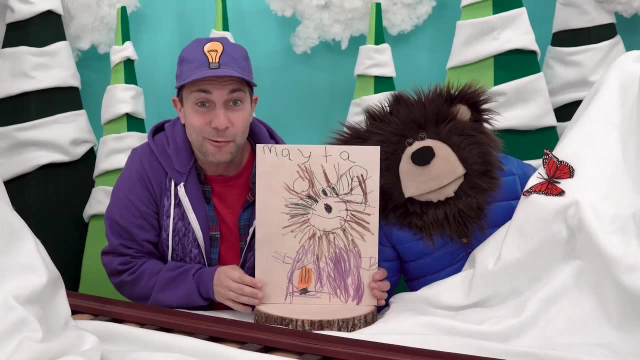 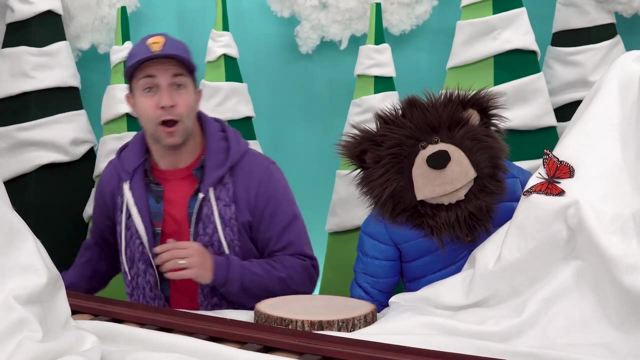 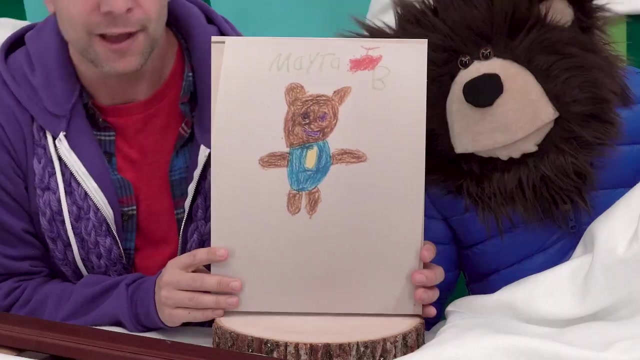 like the idea light bulb you made right here. oh, and made to look. your name is at the top: m-a-y-t-a. wow atreyu. thank you for sending us your fantastic artwork. are you ready for another piece of art? yes, look at this picture. this art was sent to us by a family in southeast asia, an amazing kid named. 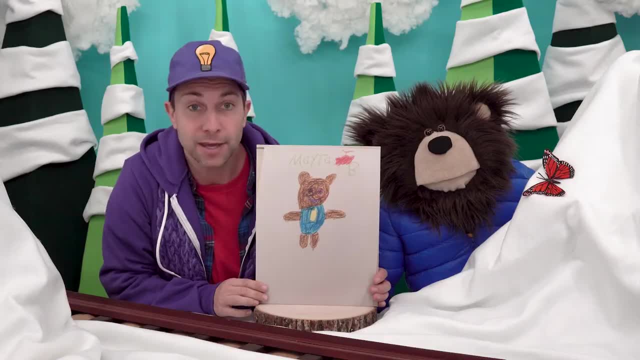 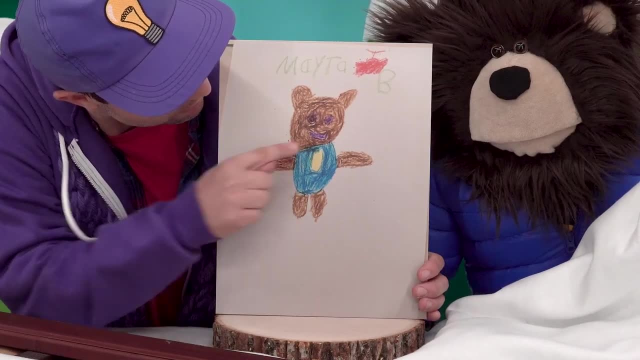 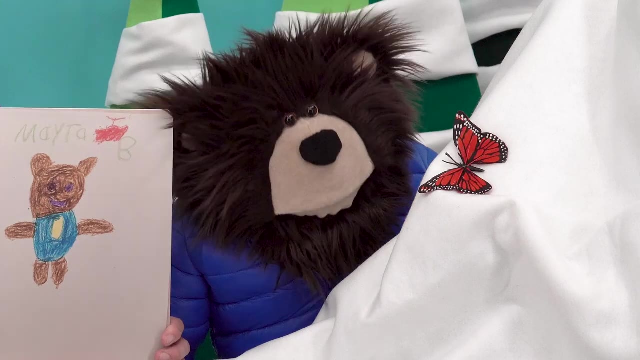 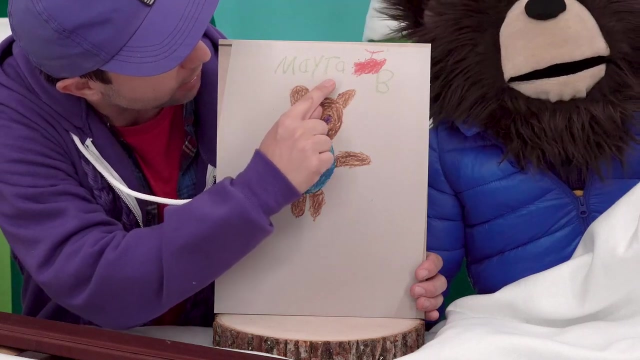 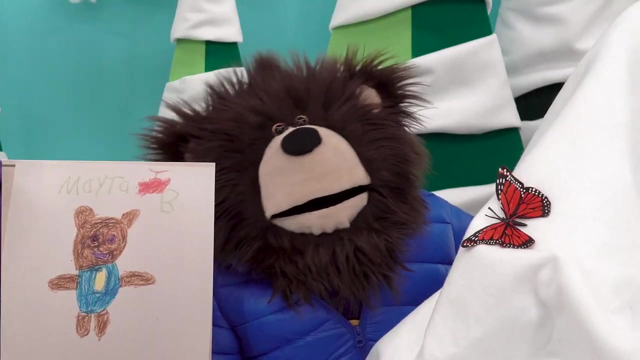 damia drew mate right here. damia, you did a fantastic job at coloring oh, and made to look. you have a little happy smile right on your face and up here is mr butterfly damia. great job at coloring mr butterfly orange. and look, there's your name: mayta, m-a-y-t-a and b. oh, that is fantastic. 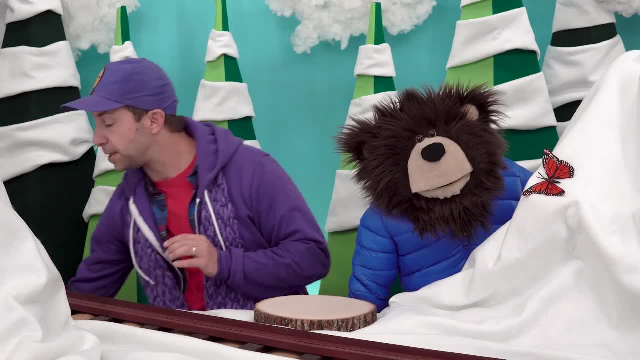 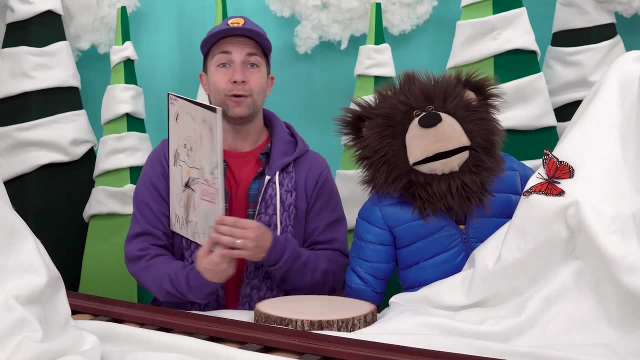 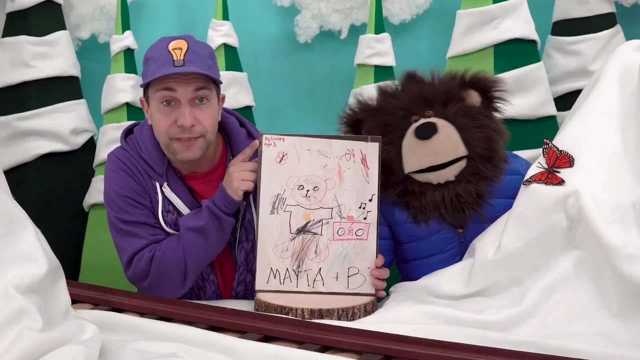 thank you, damia, for sending us your magnificent artwork, and the last piece of art that we are was sent to us by a family who lives in Canada. A cool kid named Linley made this Meta art. See. it says Buy Linley, age 3, at the top. 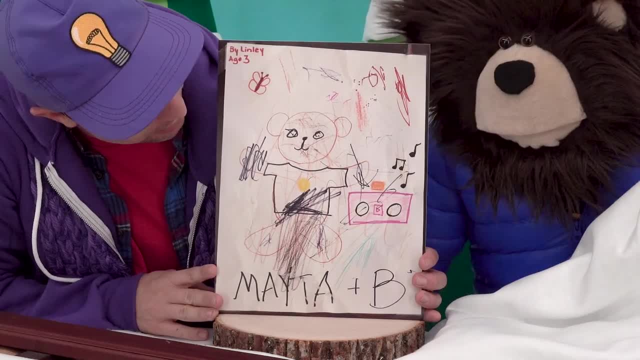 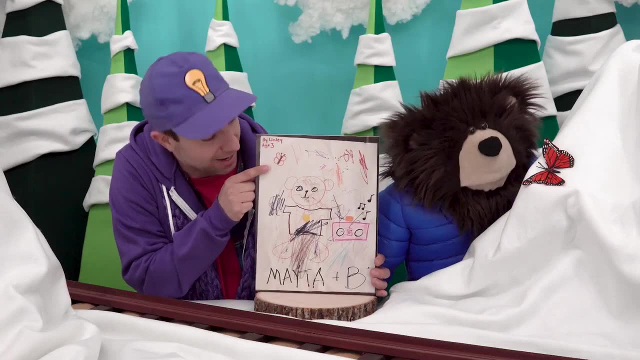 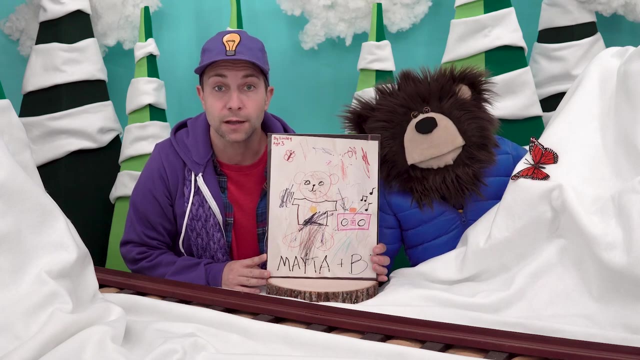 Look, Meta, there you are, And next to Meta is Pinky, the Boom Box, And flying over Meta up here is Mr Butterfly Linley. I love how you used all of these wonderful colors. Linley, thank you for sending us your fantastic artwork. 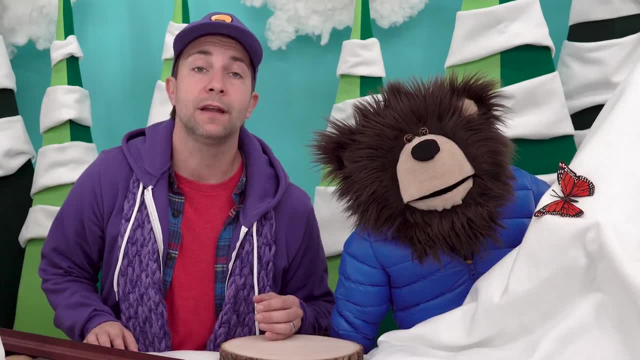 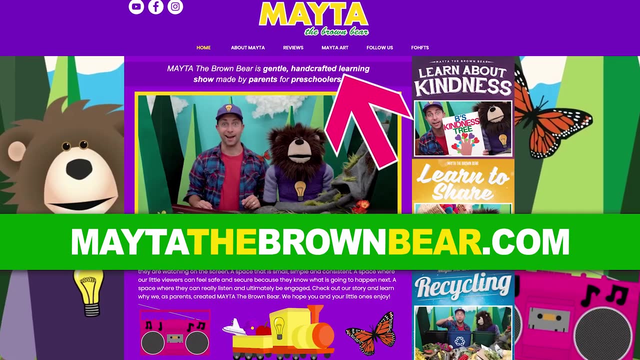 Mm-hmm Grownups. you can send us your kids' Meta art by first taking a picture of it. then go to our site, MetaTheBrownBearcom, click on Meta Art at the top, then follow these simple steps here. 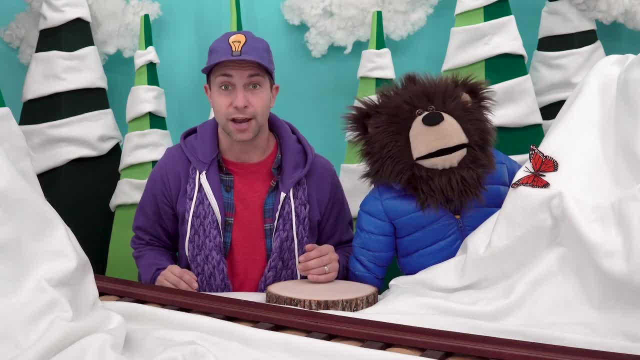 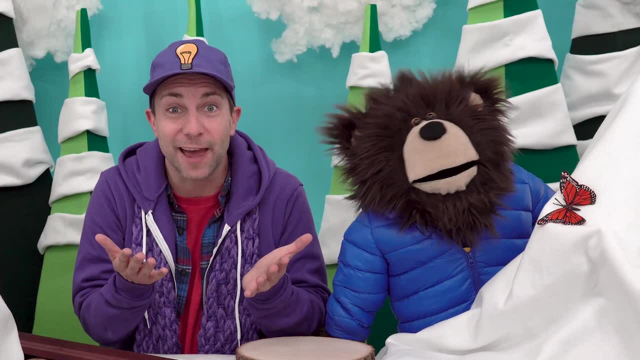 Every episode, we will print a few pieces of art and share them here Before we go. let's say five good things about ourselves. Do you want to do that? Mm-hmm? Okay, I'll go first and then you repeat what I say after me. 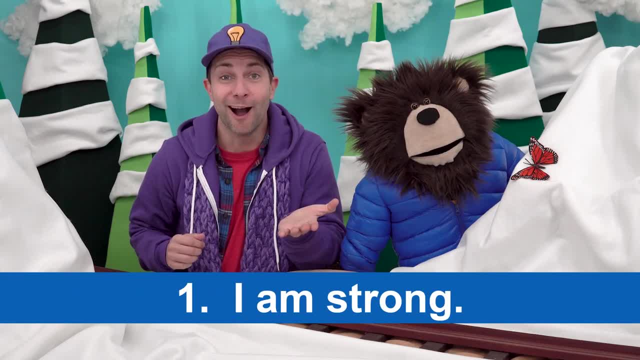 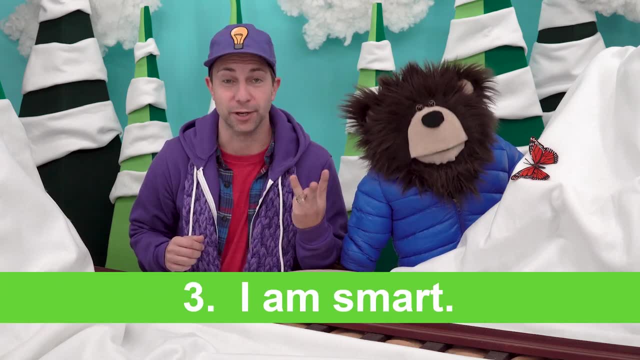 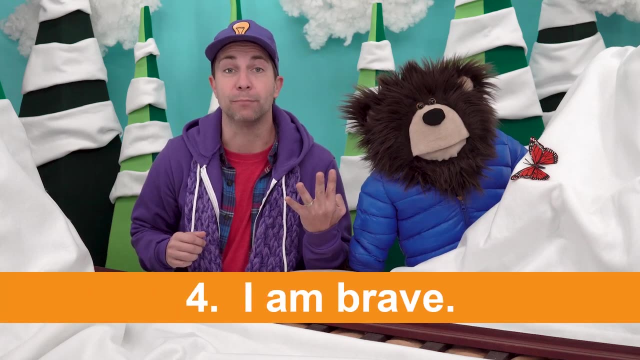 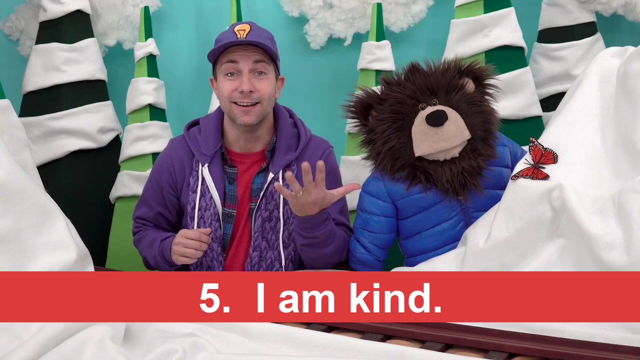 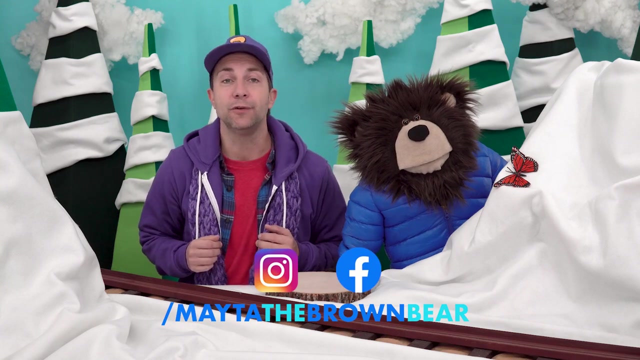 Number one: I am strong. Number two: I am helpful, Mm-hmm. Number three: I am smart. Number four: I am brave. Number five: I am kind. That was great Grownups. remember to follow us so you know when we post a new video. 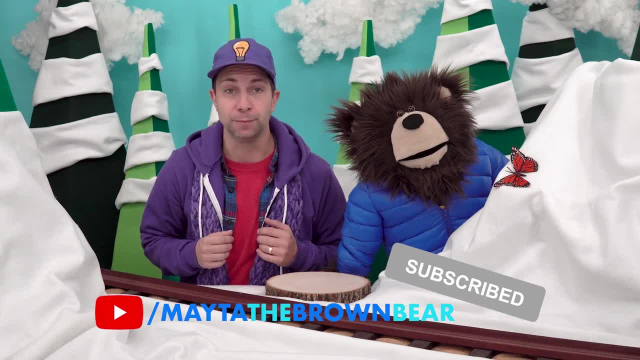 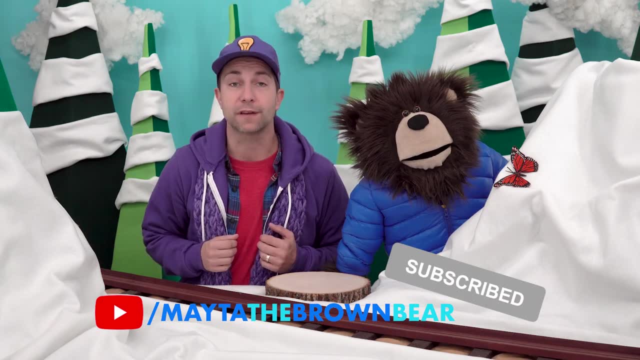 Mm-hmm, And please support our channel by subscribing here on YouTube. It's the best way to let us know you are enjoying our content. Subscribing also helps others discover our show, Mm-hmm. Go ahead, Push the subscribe button. 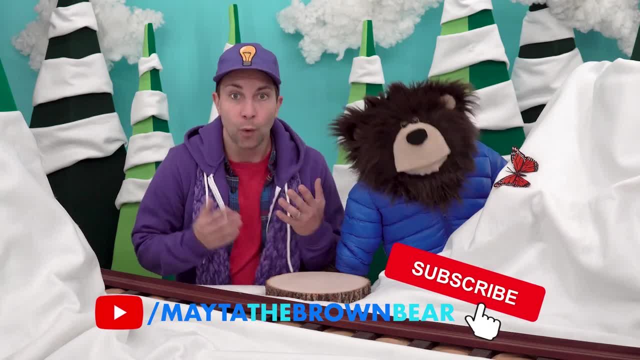 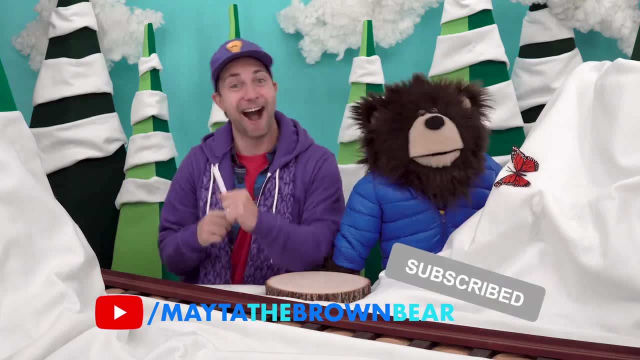 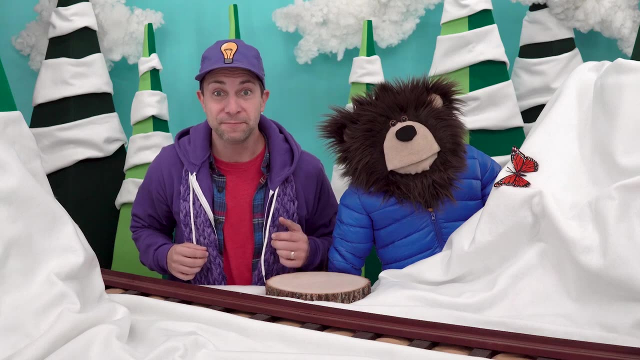 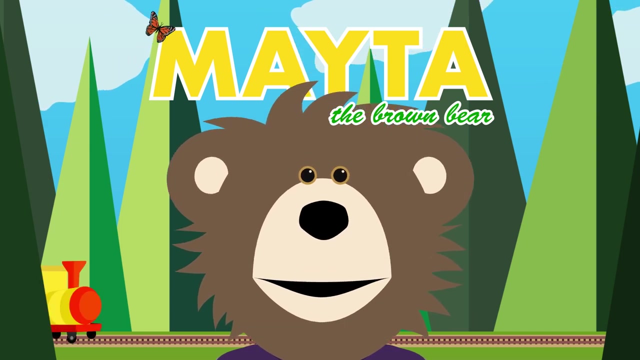 Mm-hmm, Meta and I will wait. We'll do a little dance while you print. Push the subscribe button. Thank you for spending your time with Meta and myself, And until next time. bye, Bye, Meta, Meta Meta. The Brown Bear.